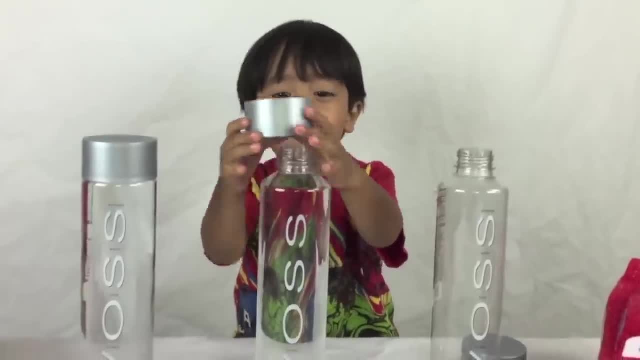 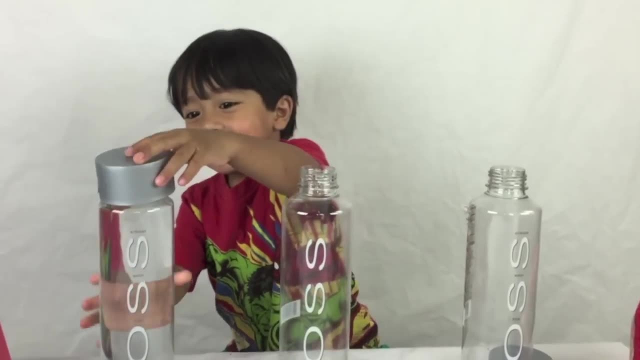 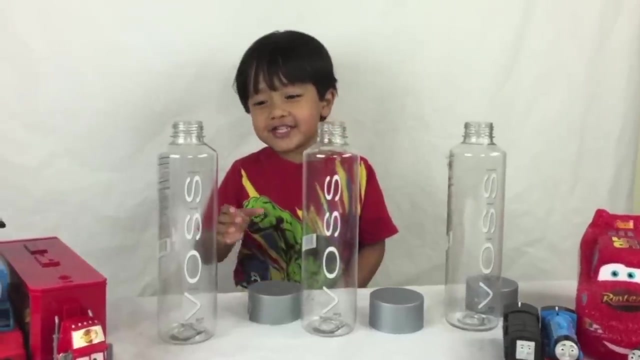 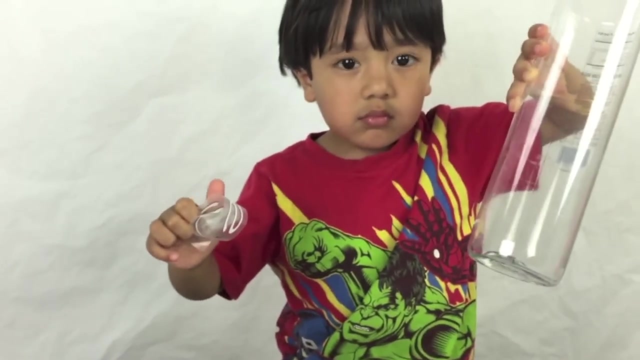 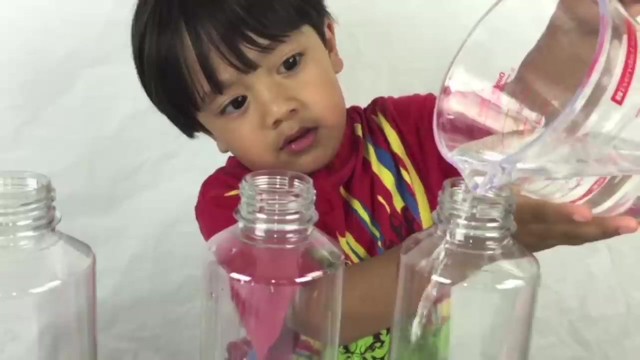 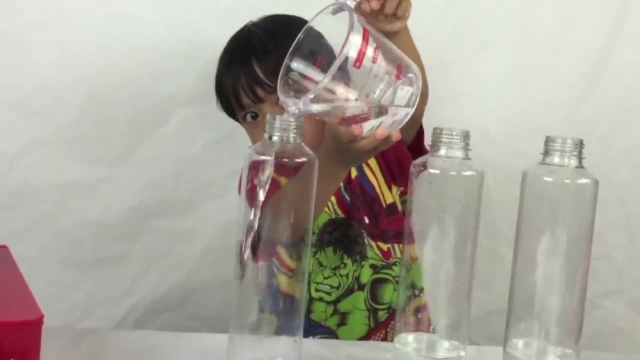 One done, Here comes the second bottle. Ugh, I'm getting full. One more left All done. Now I have to peel off the sticker. First, I need three fourth cup of water. I'm going to add Disney cards inside the bottle for fun. 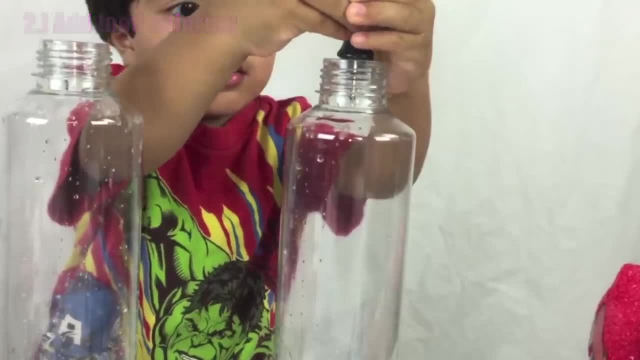 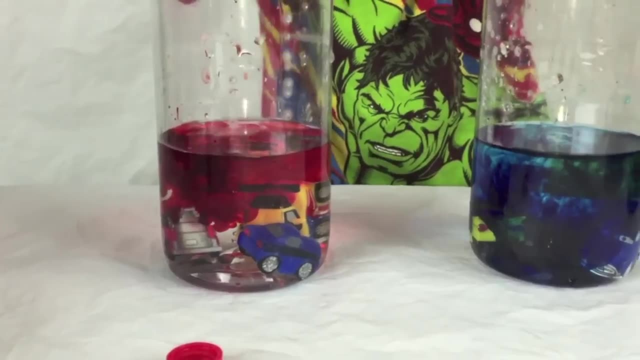 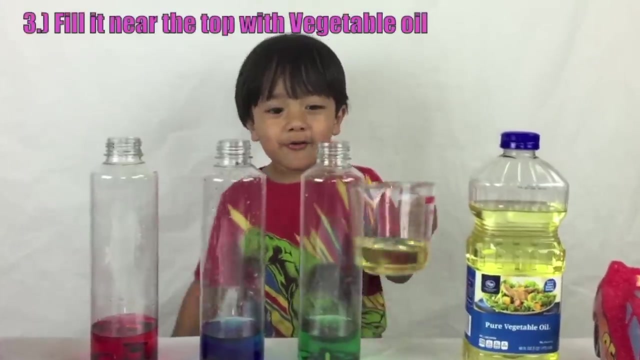 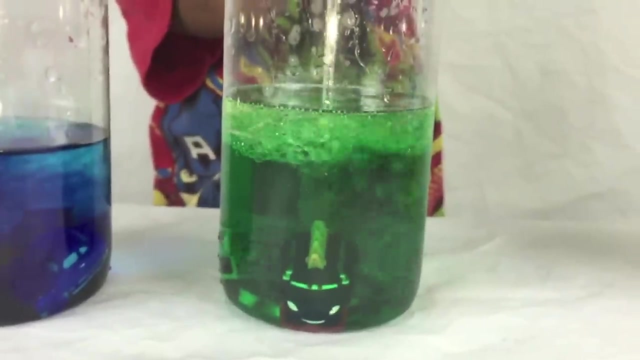 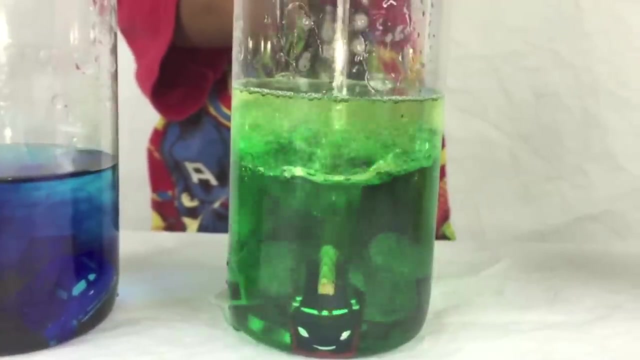 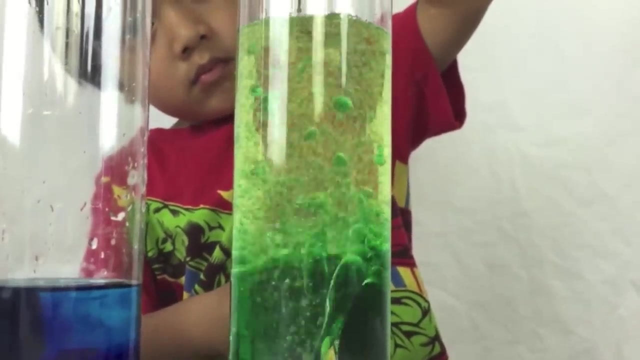 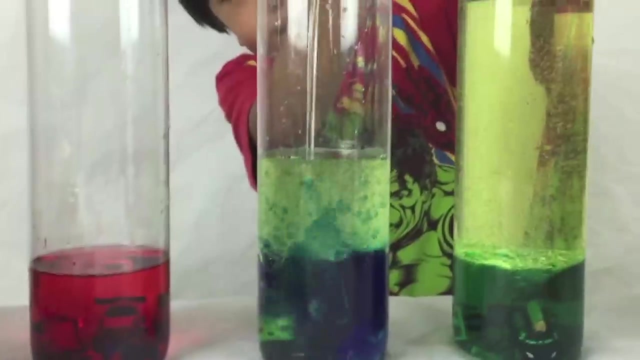 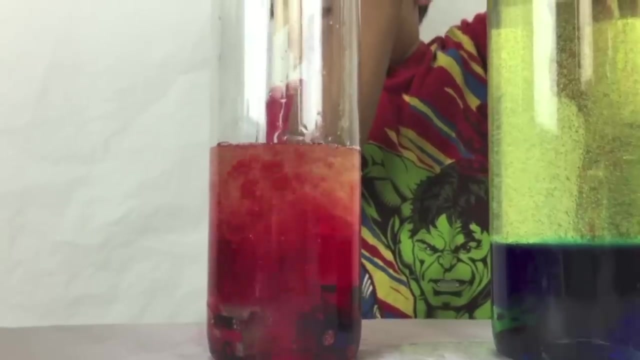 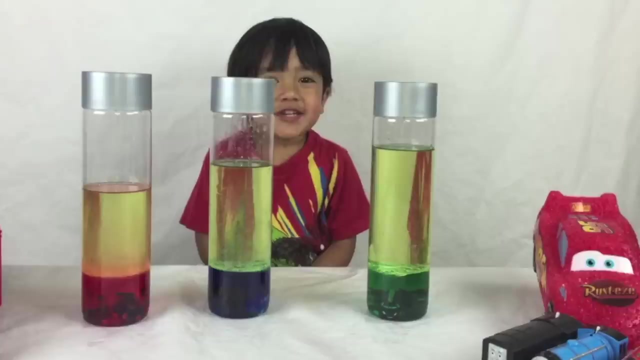 I'm going to add food coloring. I'm going to add food coloring. I'm going to add food coloring. Woah, This looks cool. All right, Let's add vegetable oil. Look at all the bubbles. Ah, This looks cool already. 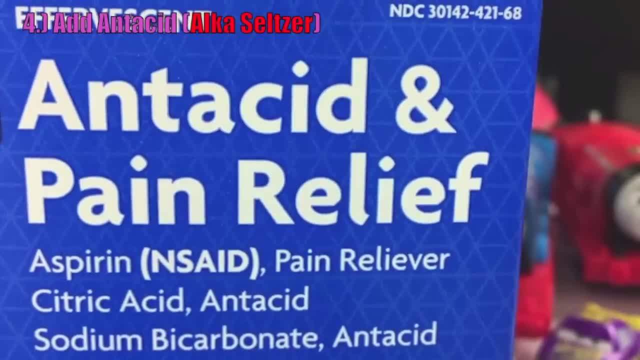 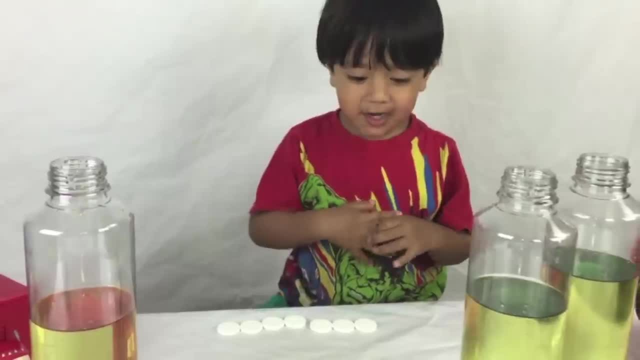 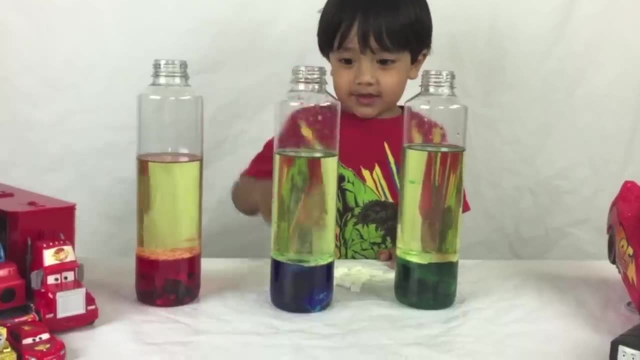 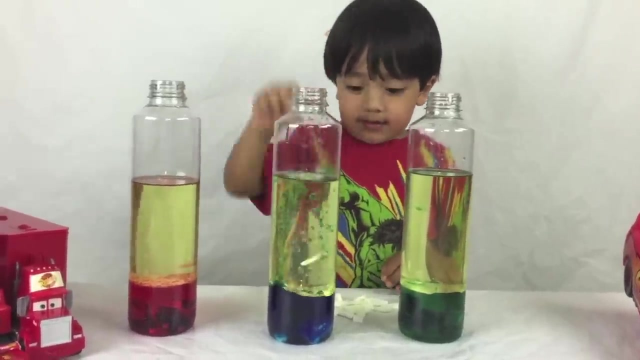 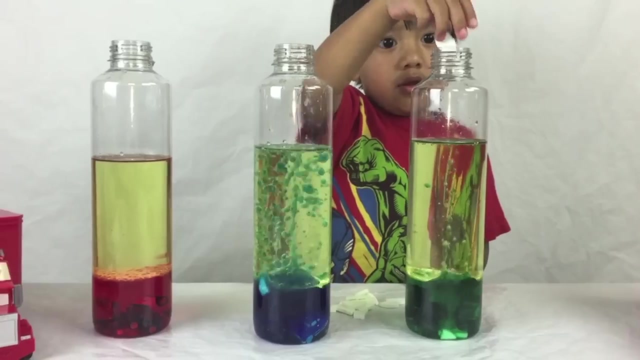 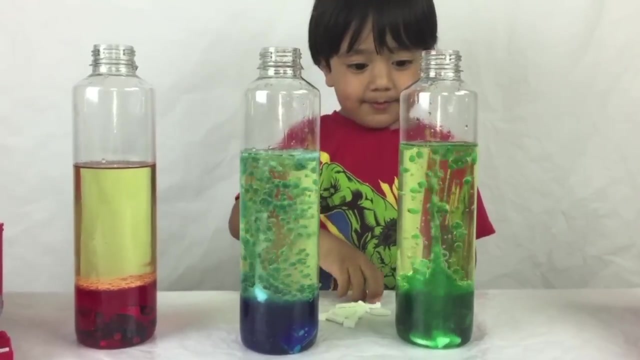 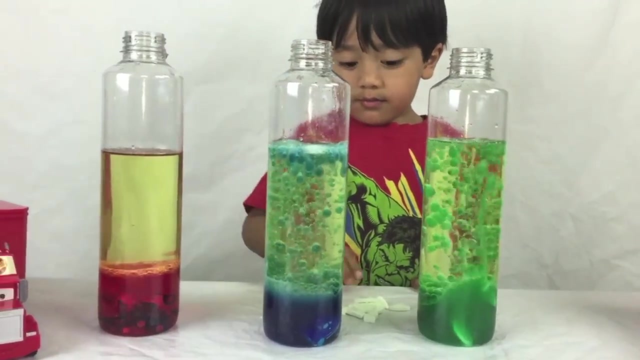 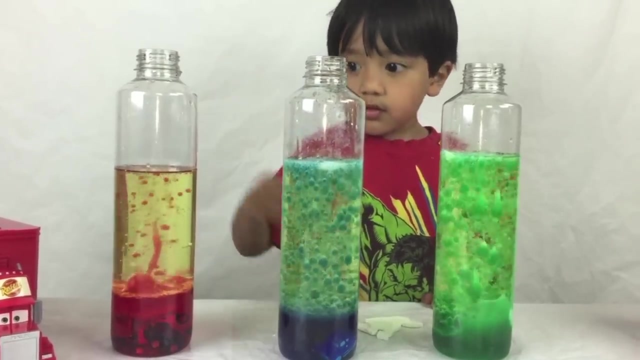 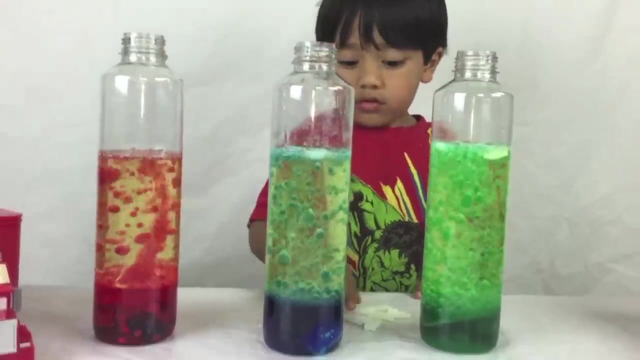 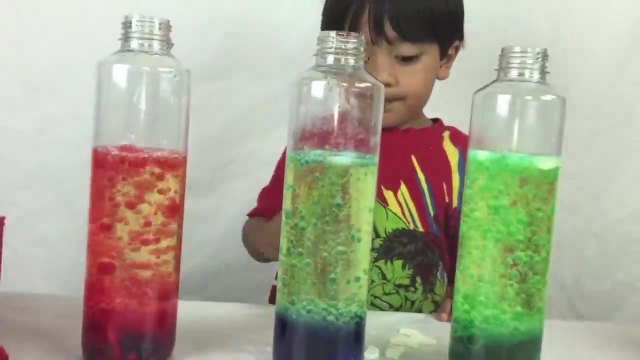 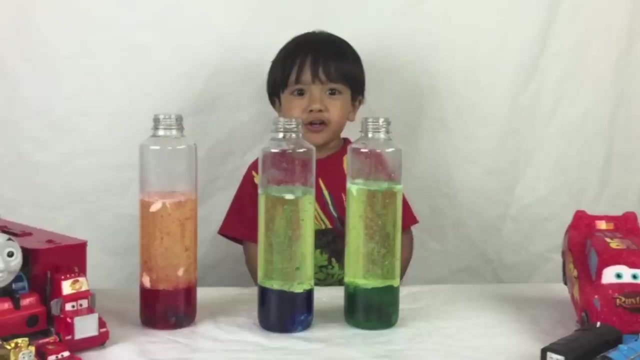 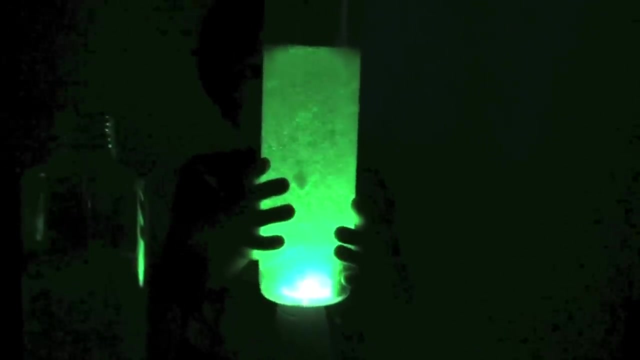 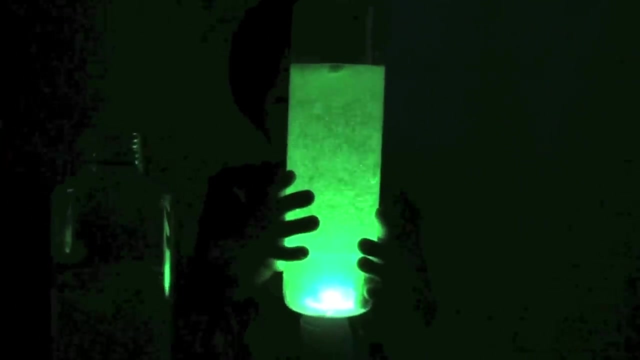 Now we have to add Ant's Axe. Next I'm going to break them in half. Trains and Cars are ready and enjoy the show. I like all of the bubbles, I know. Turn it off and use the flashlight. I hope you like the ride. 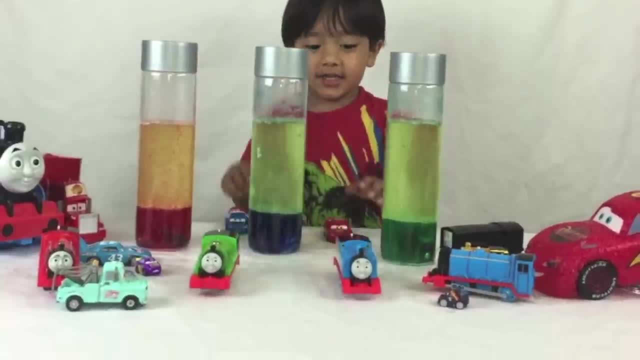 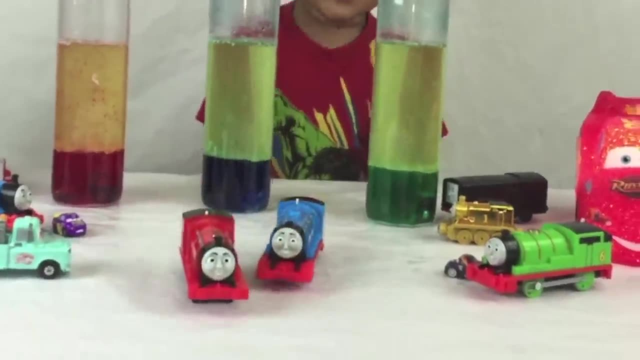 Thanks for watching. Go, make your own Go race. Oh, Thomas is winning. I think they both won. I think they're going to fall. Oh, James is winning. He won, James won, Yeah, he did. 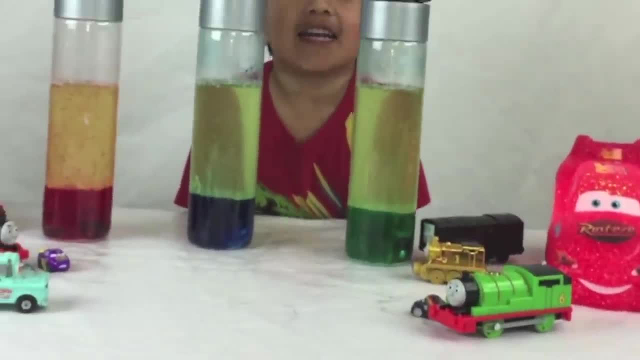 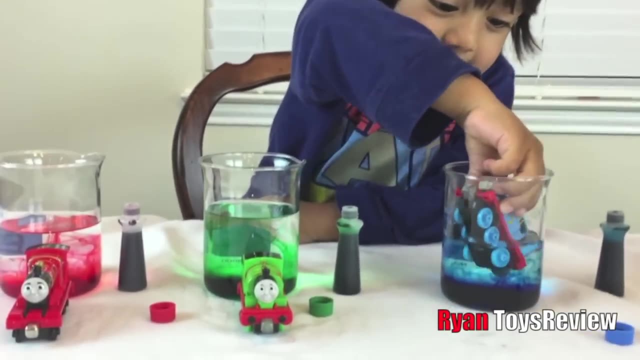 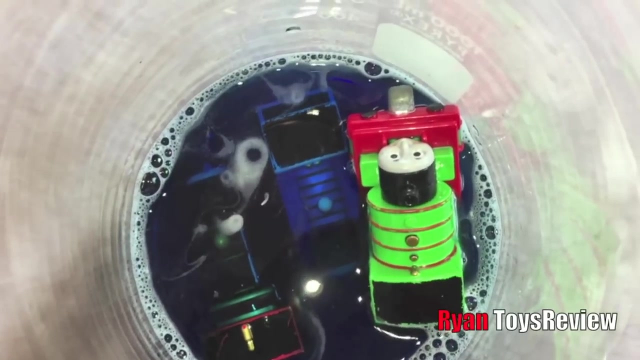 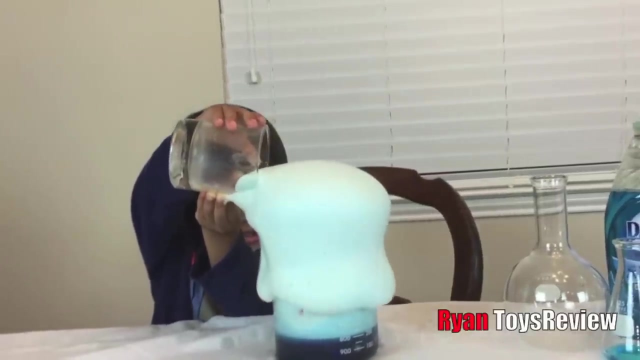 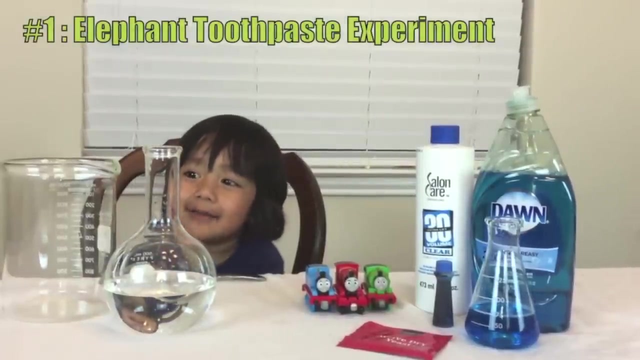 Hey Ryan, Hi Mommy, What are we going to do today? I'm going to play experiment, Experiment. 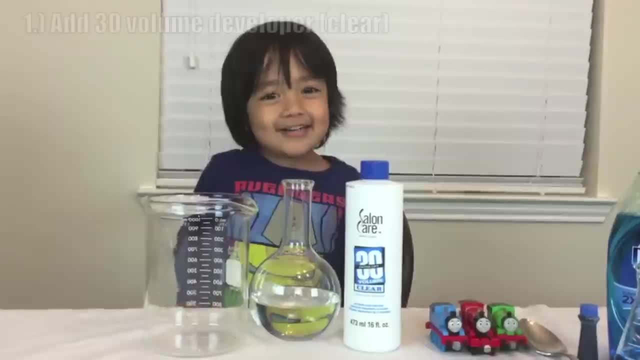 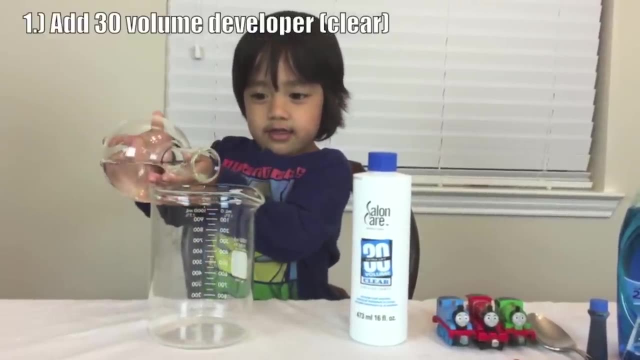 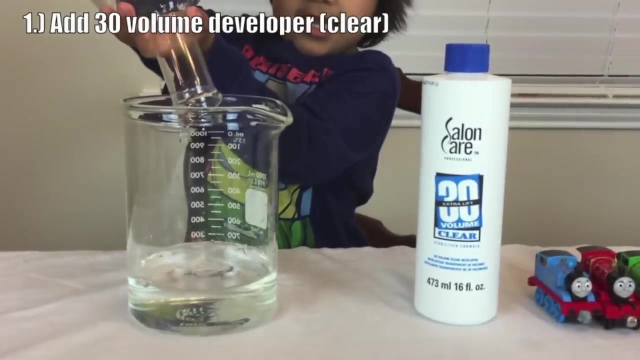 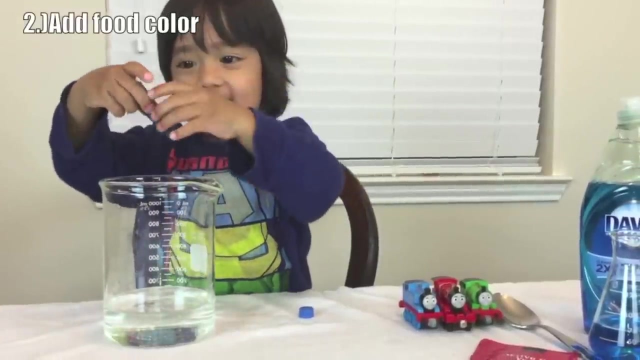 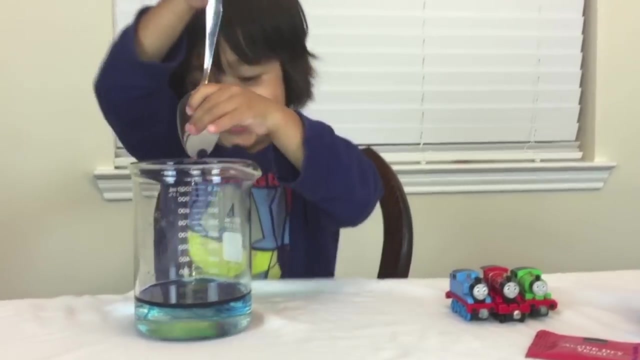 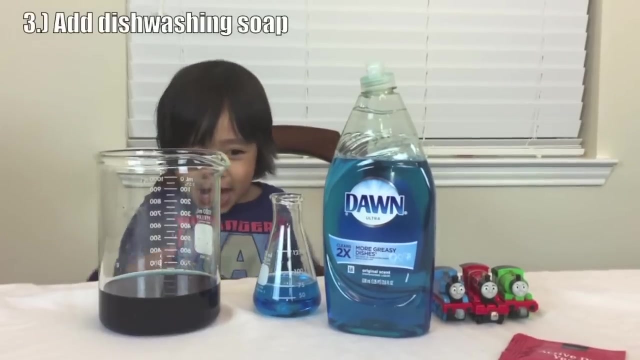 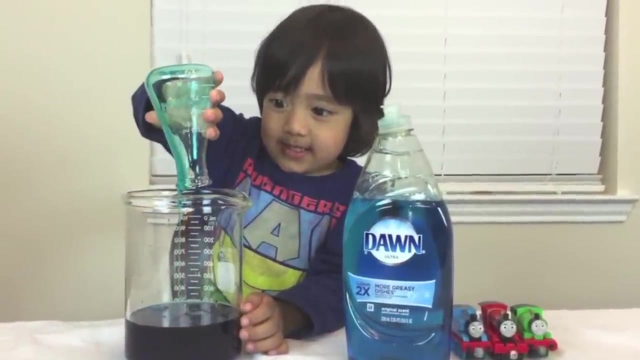 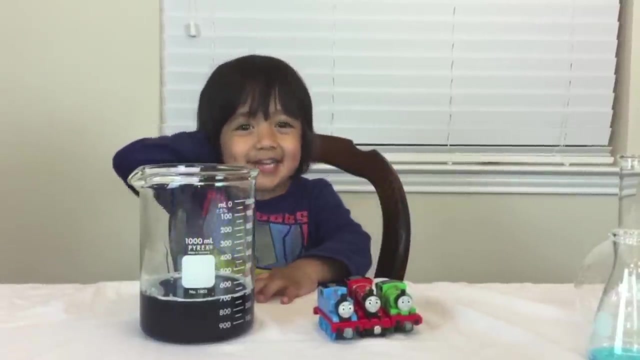 That sounds super fun. I'm going to color it blue, I'm going to stir it And now I'm going to add Dawn's salt. I'm going to put Percy and James and Thomas inside the beaker. 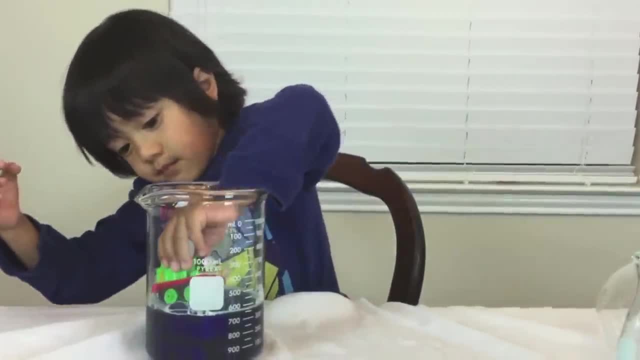 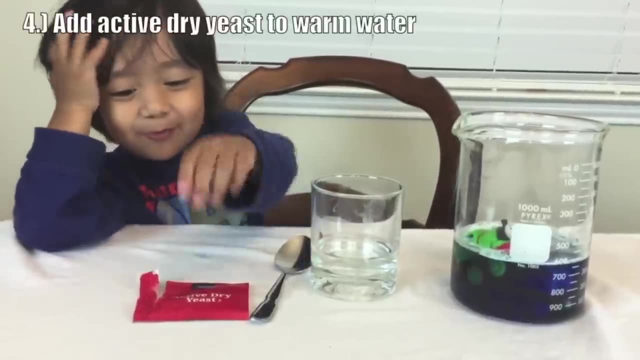 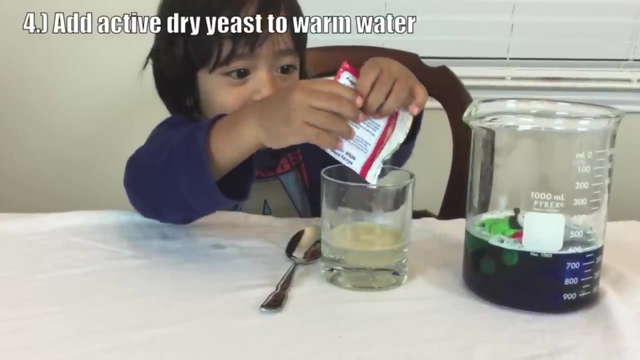 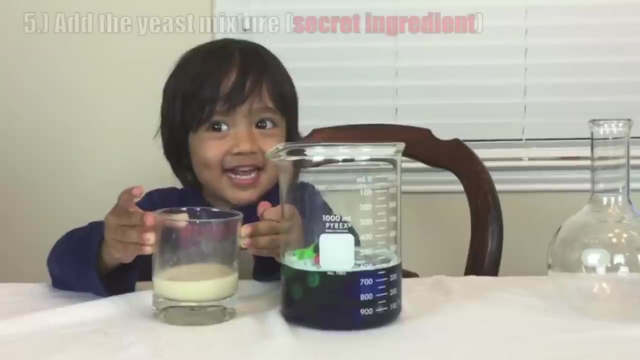 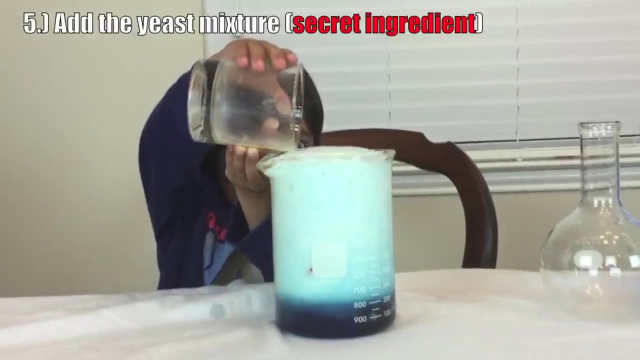 Now I'm going to add yeast inside the warm water. Now I'm going to mix it together. Now I'm going to sieve it and clean it up. Now I'm going to mix it together, Mix it together, Mix it well until you're done. 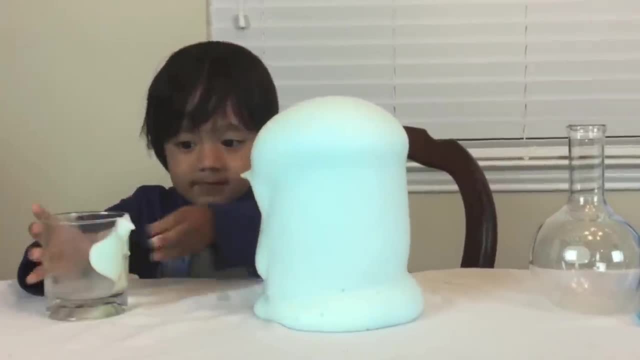 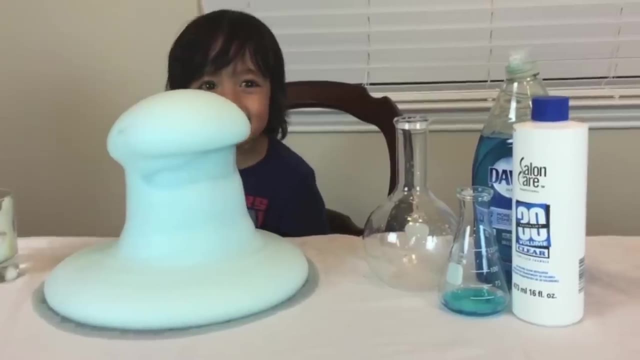 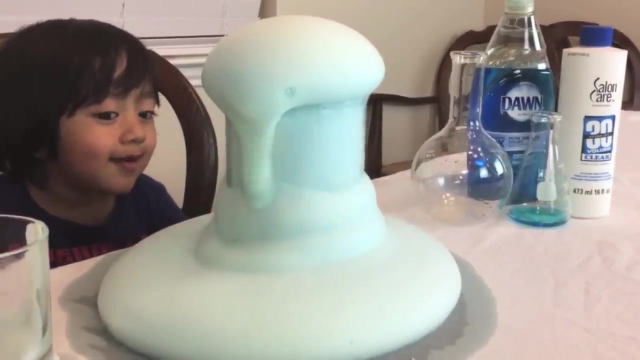 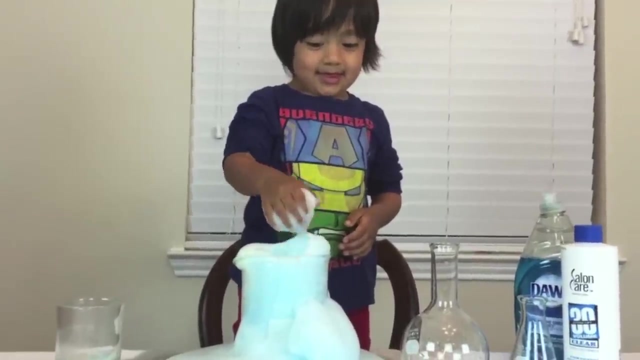 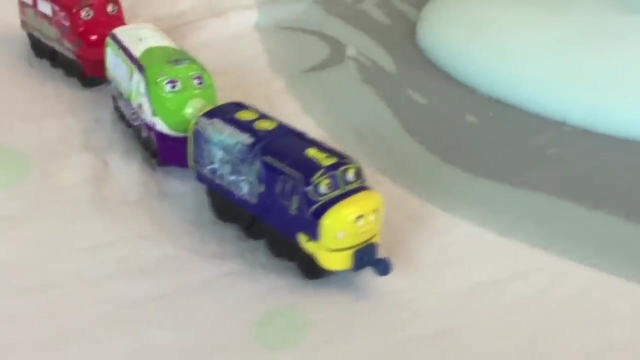 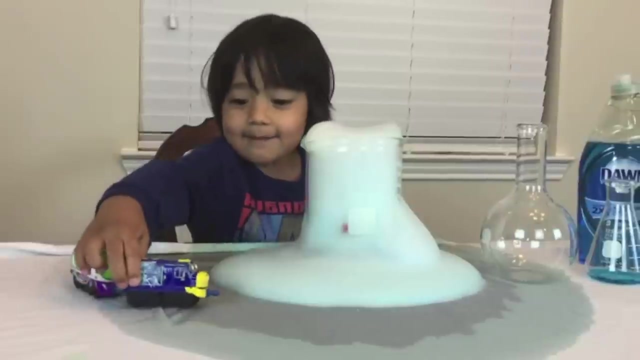 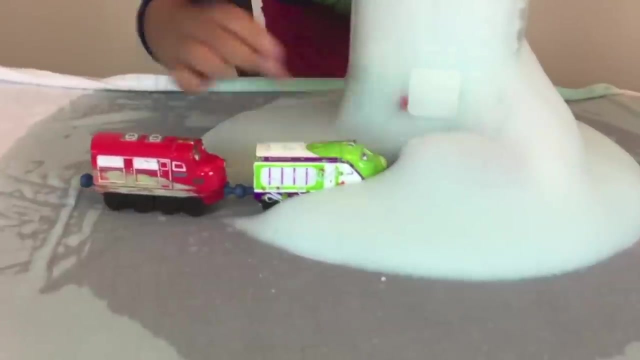 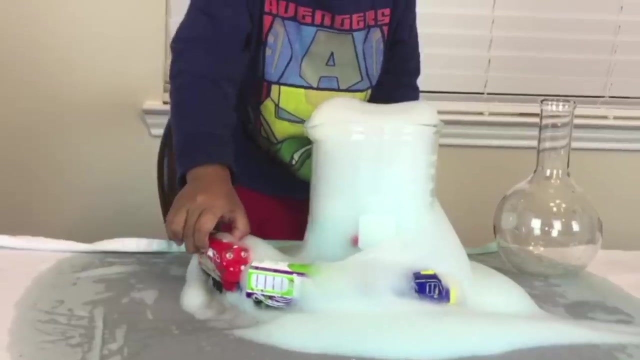 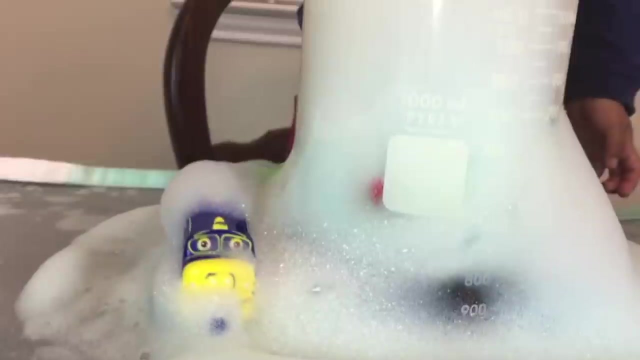 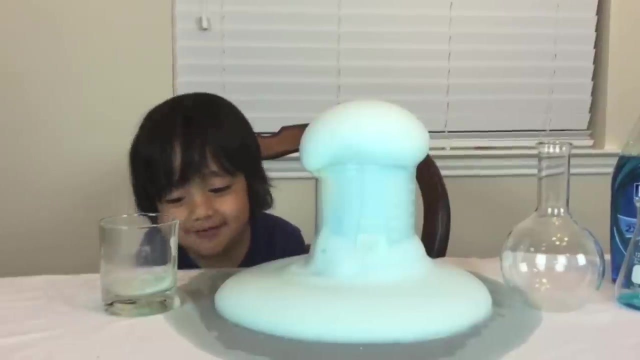 Mix it, Mix it, Mix it well, Mix it well. Wow, Wow, Okay, Ryan, put it down. Wow, Wow, Okay, Ryan, put it down. Wow, And then enter the following: That was fun. let's do another experiment. 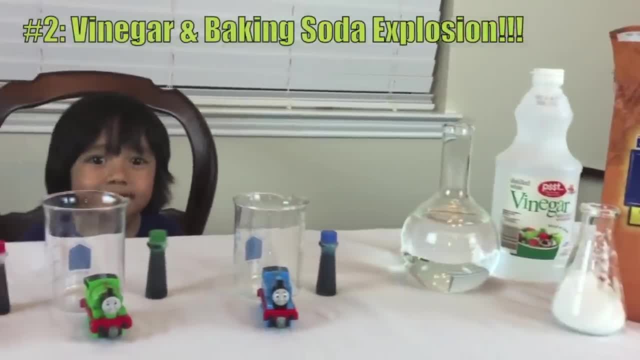 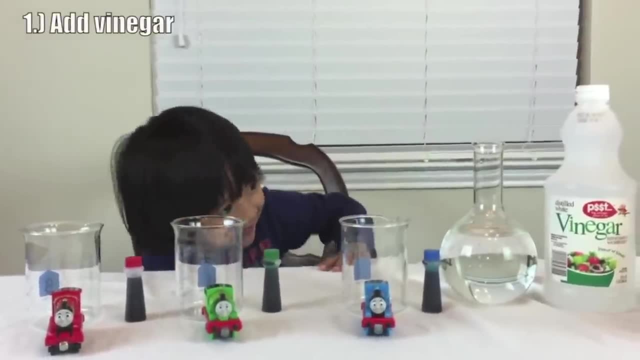 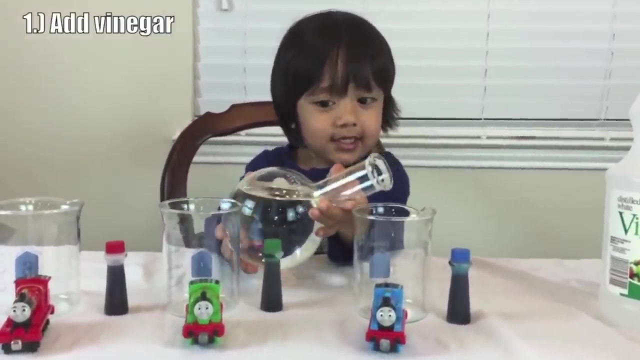 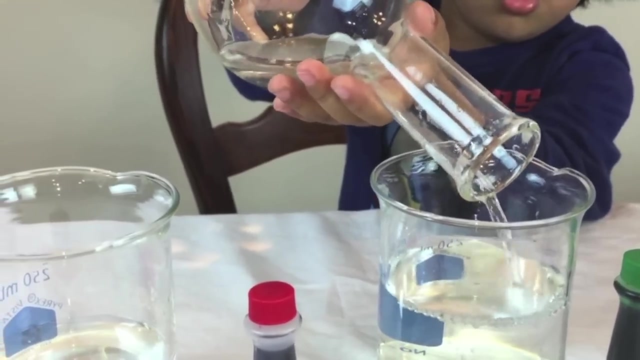 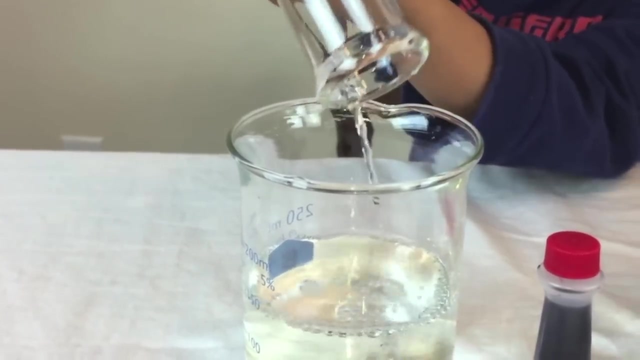 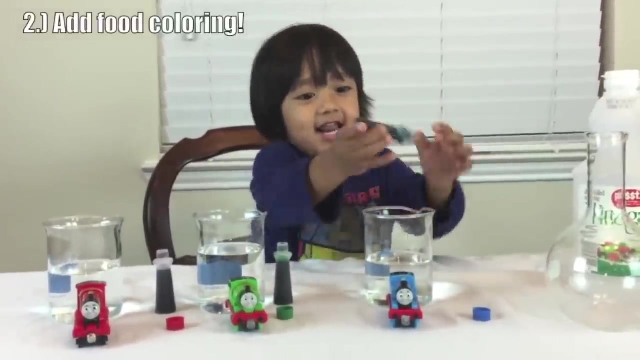 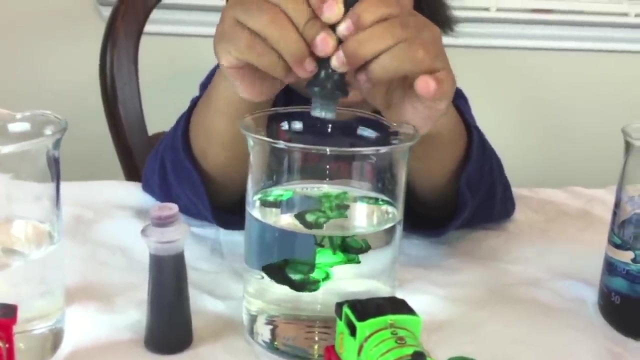 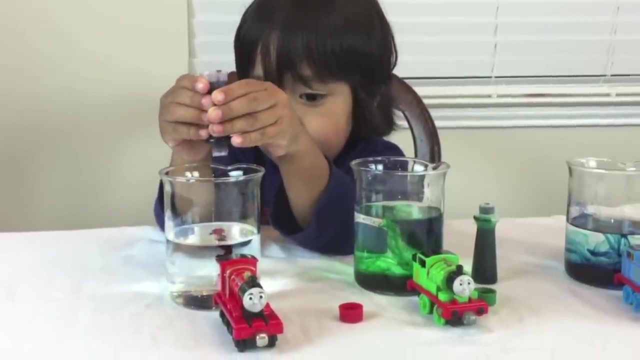 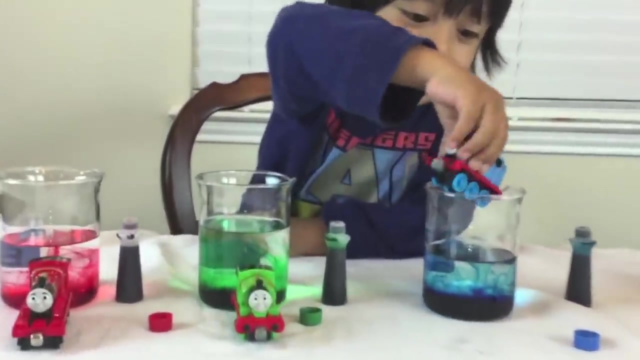 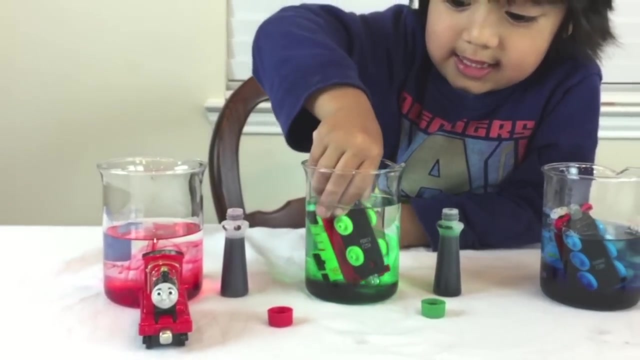 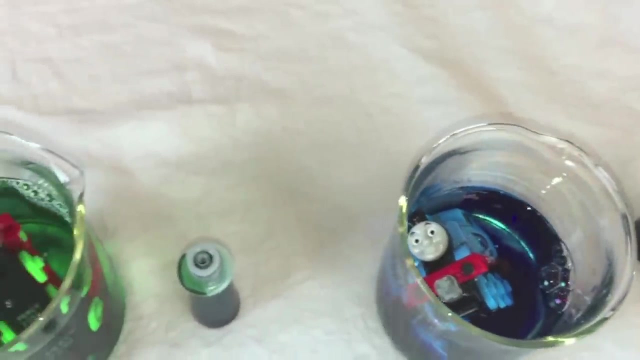 That was fun. let's do another experiment. I'm going to put the vinegar inside the beaker. Now I'm going to color the vinegar. I'll put two in here And go: Thomas and Percy and James. Now I'm going to add baking soda. 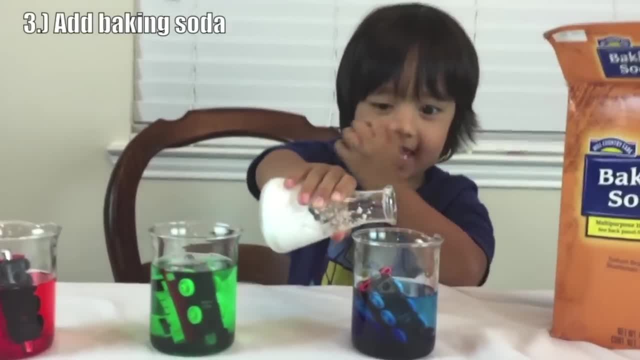 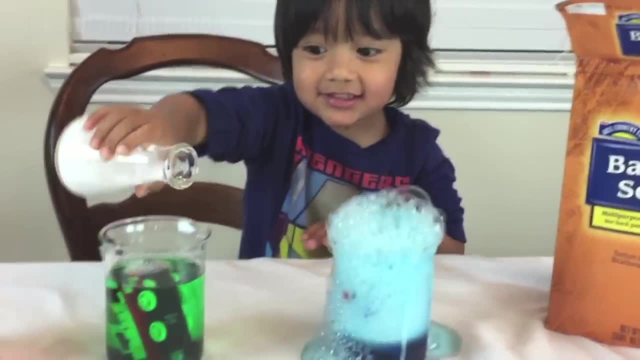 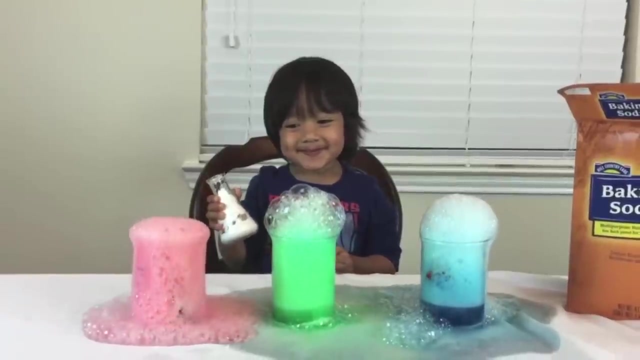 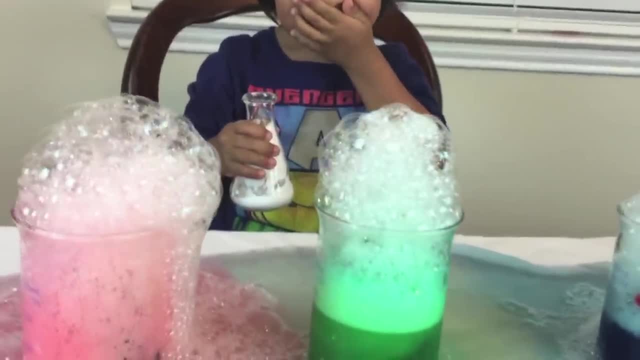 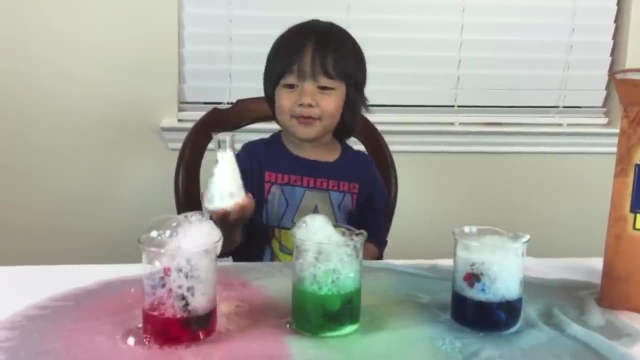 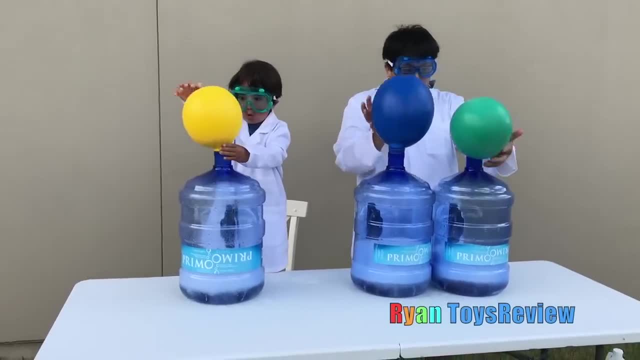 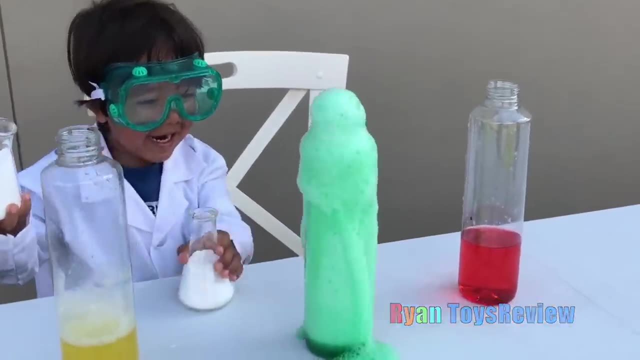 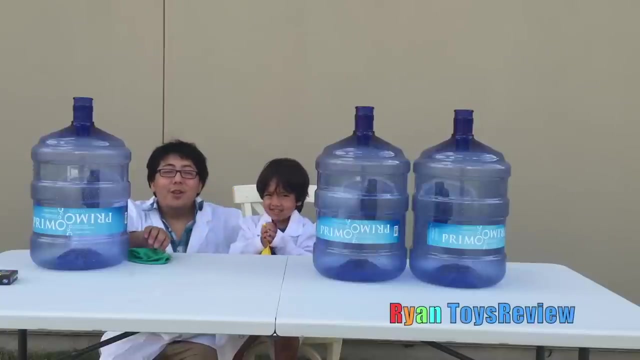 Whoa, Whoa, Whoa, it's blowing up Explosion. Welcome to Ryan ToysReview. Hi kids, Today we're going to do a science experiment with baking soda and vinegar, Blowing up giant balloons. First, we need to add vinegar. 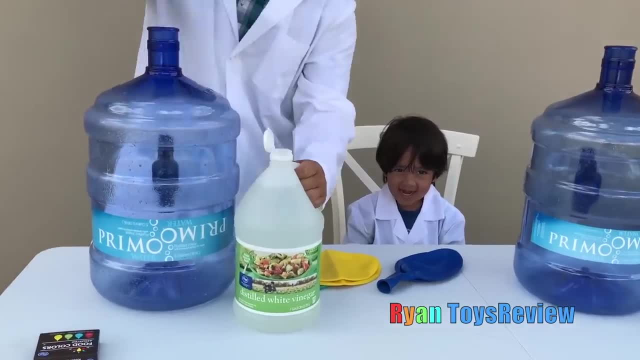 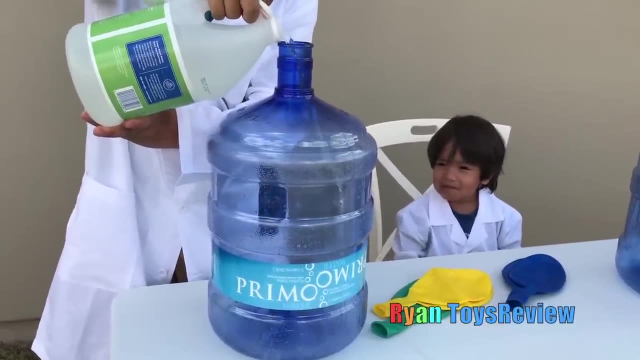 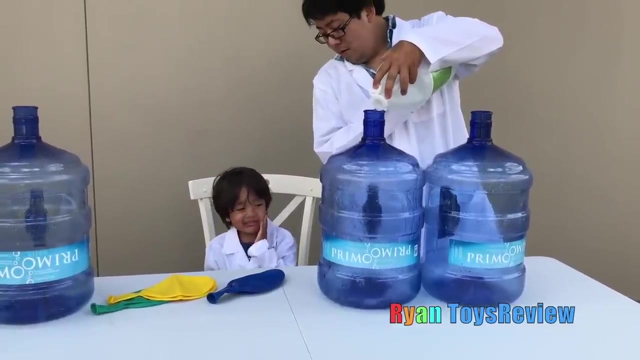 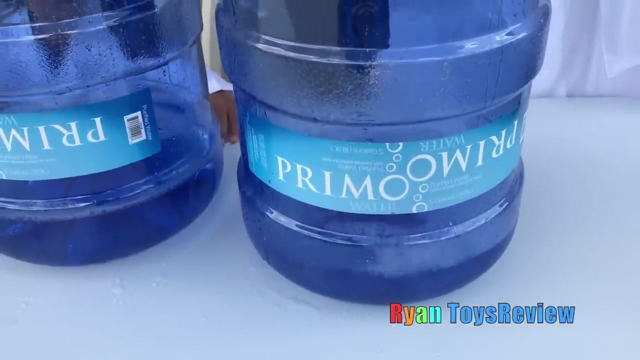 And this: Let's put that in a container. Ooh, smells. Alright, ready, kids, Kids. it looks like water. Let's add it to the other container too. Last one, Next, put baking soda into the giant balloon. 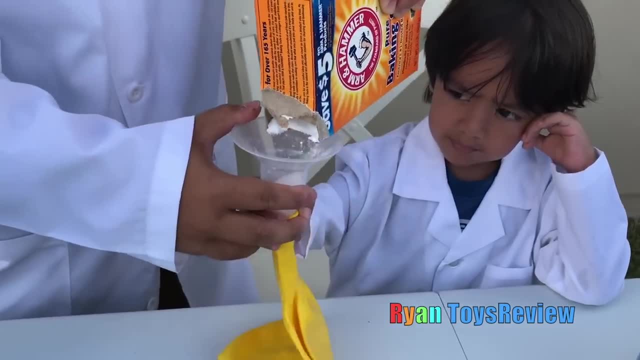 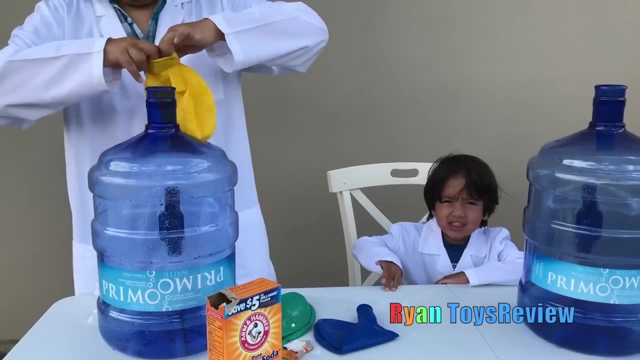 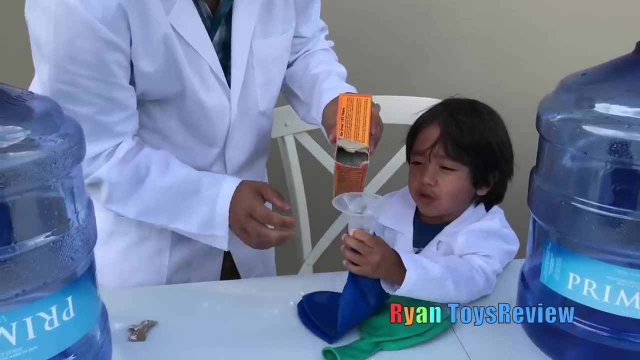 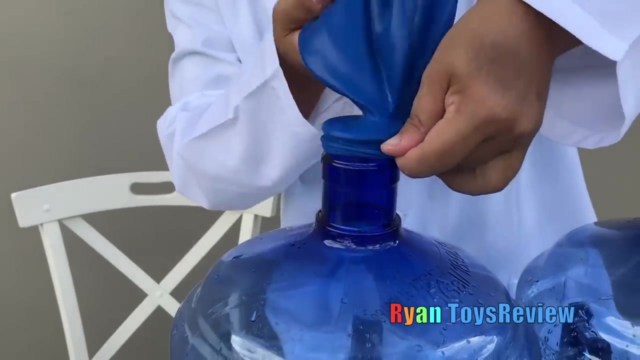 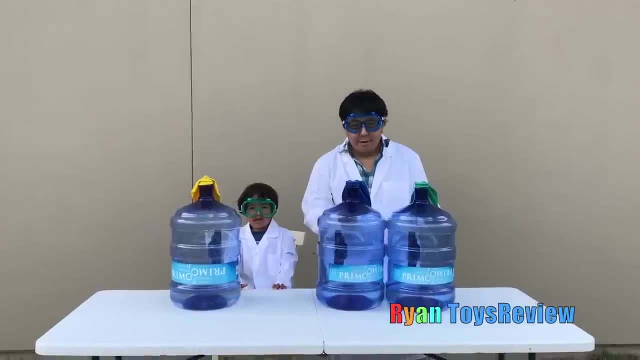 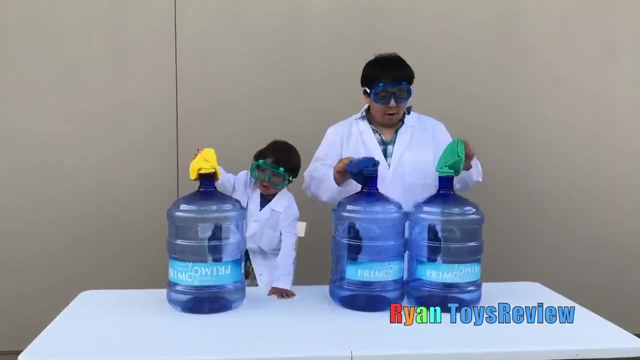 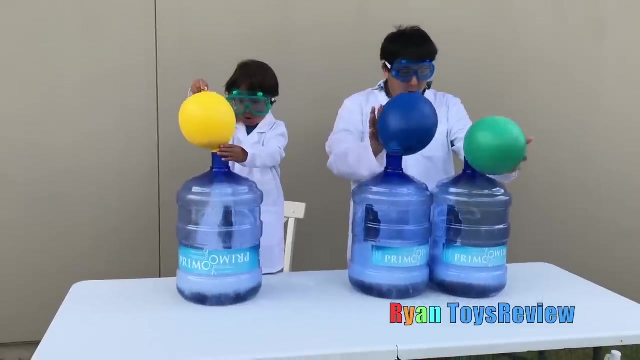 Shake it, shake it, shake it. Now that we got our goggles on, let's put the baking soda into the vinegar. Let's do it Three, two, one go, Whoa, whoa, whoa, Whoa. it's blowing up. 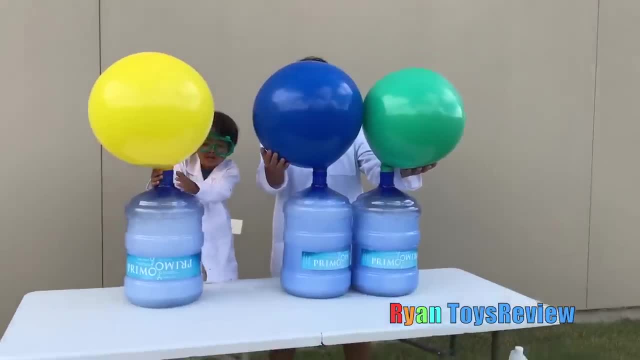 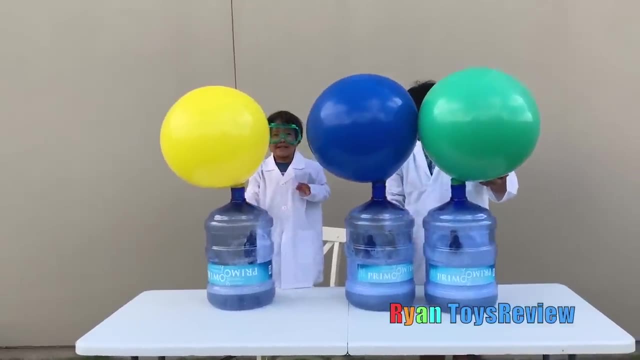 That's big. Look at this, Look at the big water. How did this happen? It's not stopping Boing, boing, boing, boing, boing, boing. I feel like it's done, It's done. 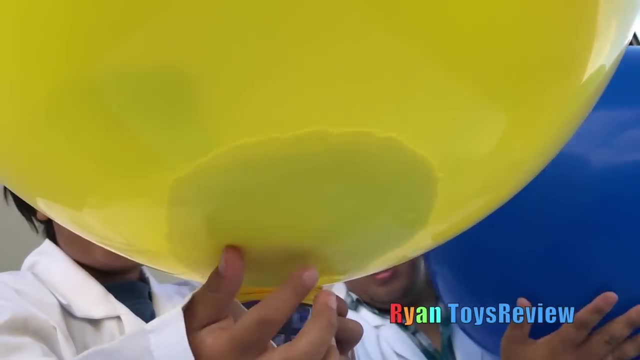 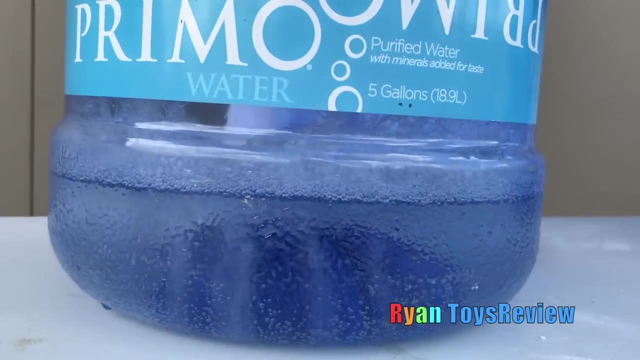 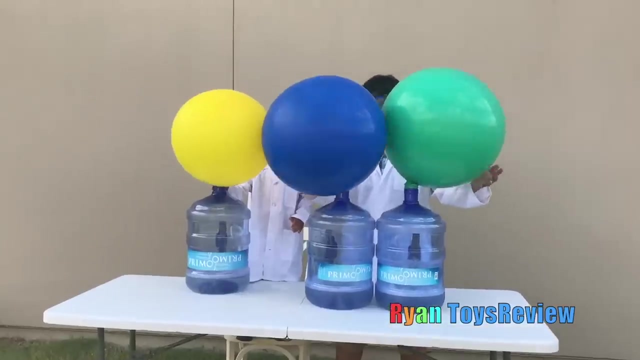 Mine's still going kids, See some in there. Cool, It's a giant balloon. Oh, it's a giant balloon. Cool Kids, that one's still going green. Woo-hoo. Alright, let's take the balloon out. 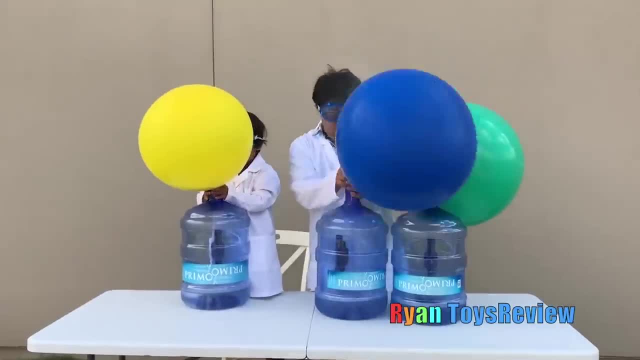 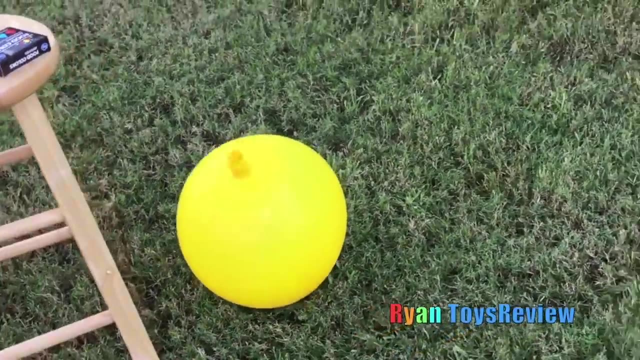 Woo-hoo, woo-hoo Ah Help. Woo-hoo woo-hoo, Woo-hoo, woo-hoo Ah, Woo-hoo Help, Woo-hoo Help, Woo-hoo Help. When they pop up, they sound like a farting sow. 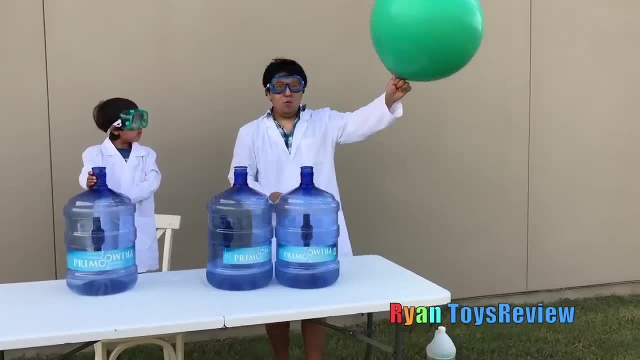 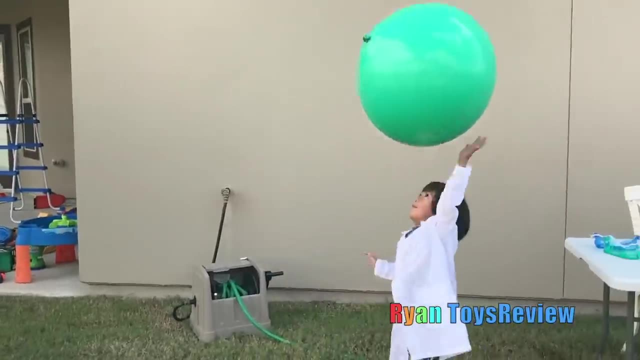 Ha-ha-ha-ha-ha. Woo-hoo, Woo-hoo, Woo-hoo. Now let's play with our balloon. Ha, Woo-hoo, Hooray, Hooray, Ha-ha-ha-ha-ha. 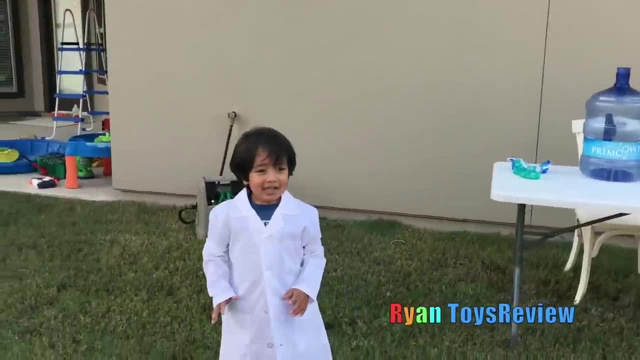 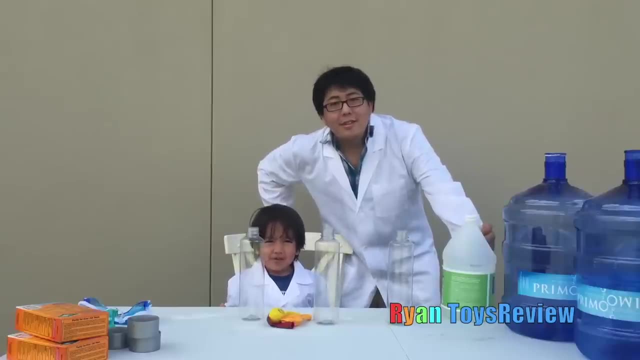 One, two, three, Ah, Kick, Woo-hoo. That's tough. Kick, Kick, Kick. Now you can do this all by yourself with smaller balloons. Yeah, like that's water bottles. Add the vinegar into the container. 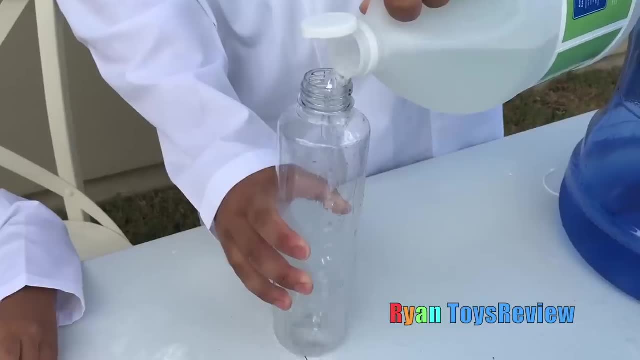 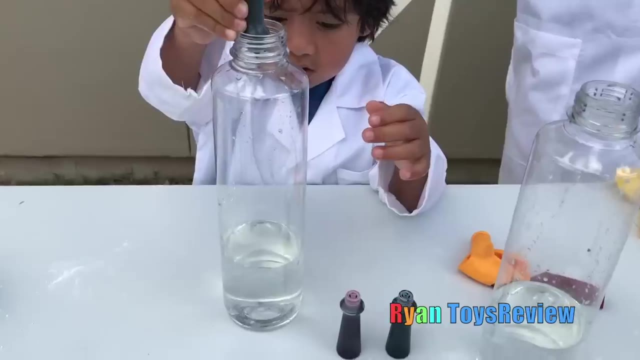 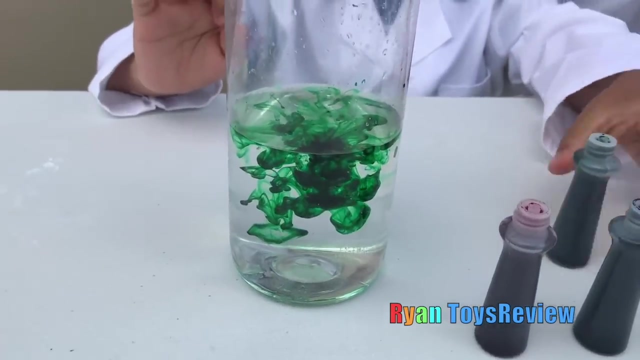 Oh, that's a lot of vinegar. Oh, that's a lot of vinegar. Oh, that's a lot of vinegar. I'm going to add food coloring into the vinegar. One, two, three. Now we're going to add blue. 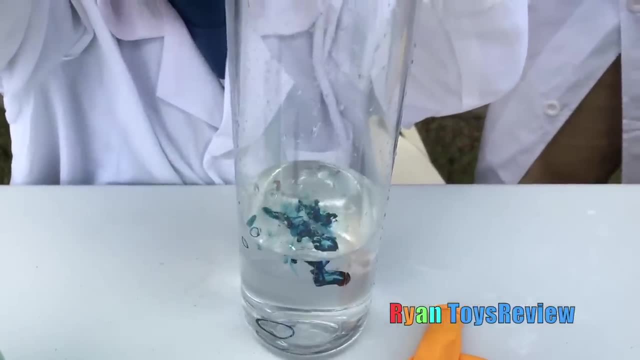 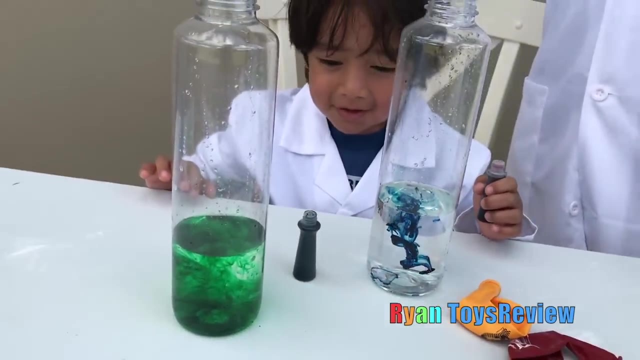 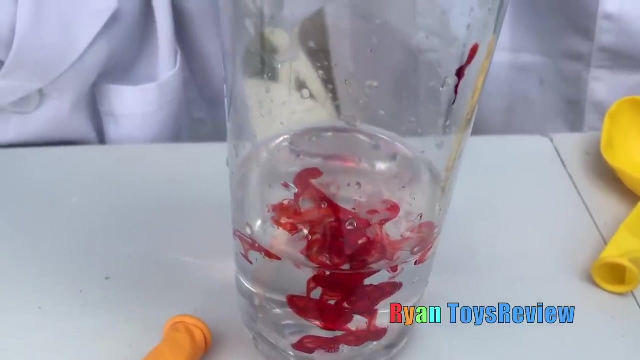 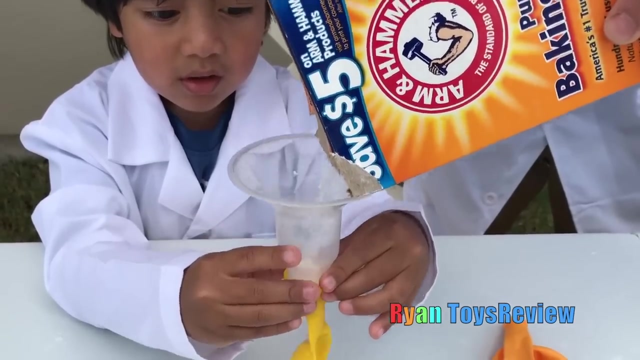 One, two, three. Whoa, look at the green one already. Try the red one, One, two, three. Good, Now we're going to add baking soda into the balloon. Now let's blow up the balloon. All right, turn it around. 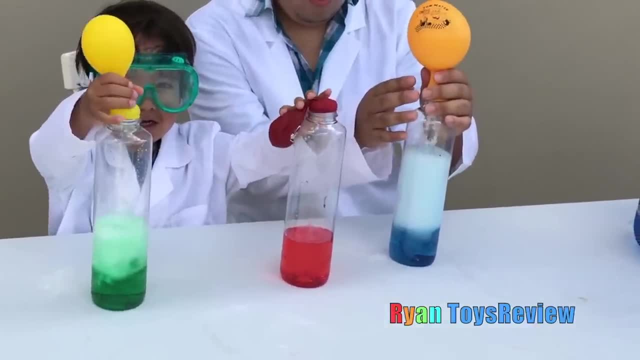 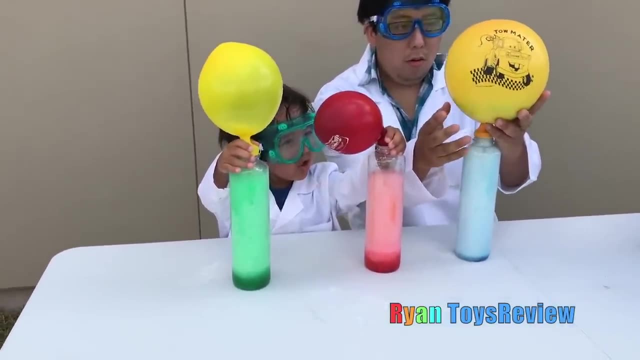 Whoa, whoa, whoa, Whoa, Whoa, whoa, whoa. They're getting big. Whoa, Look at the bubbles. They're getting big. It's getting ginormous. Look at the bubbles. 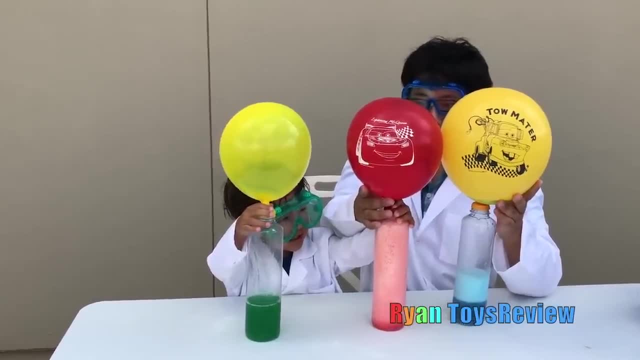 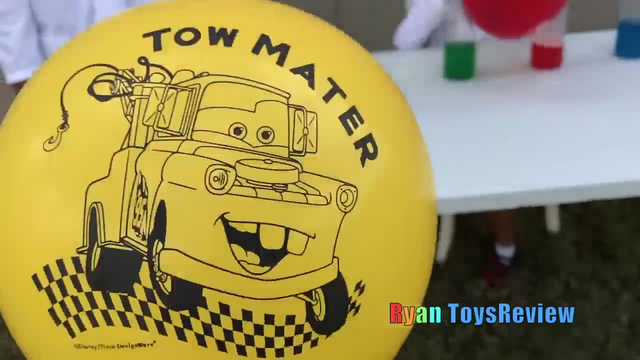 Oh, the red one is still doing it. Yeah, that was cool. Oh Whee, Hi Mater. Oh, ooh, Ooh, Ooh, It's by the balloon. All right, Now let's try it without the balloon. 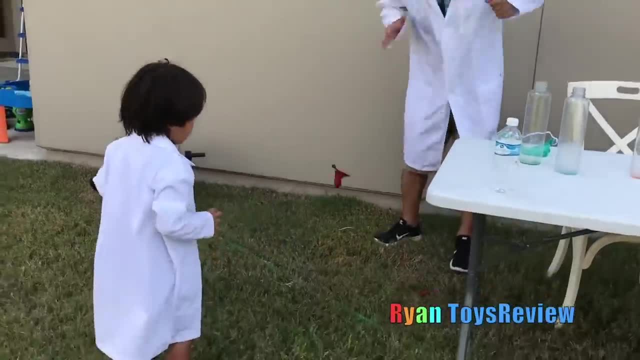 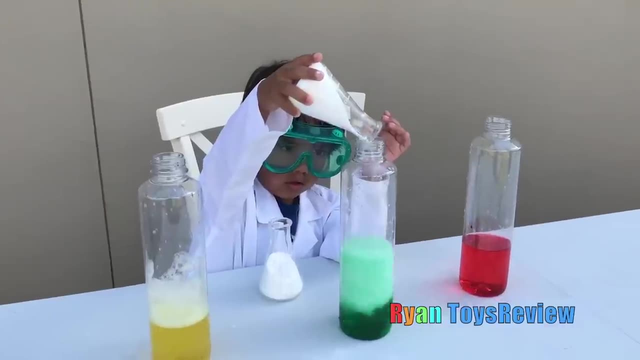 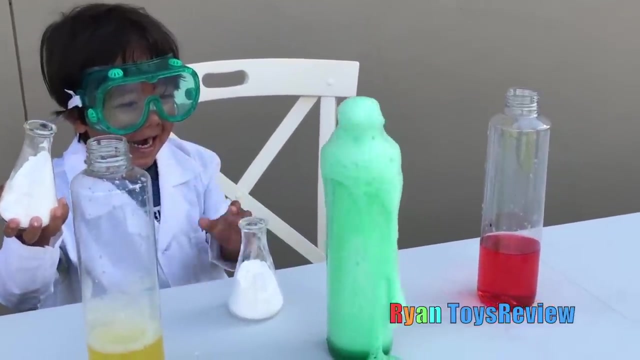 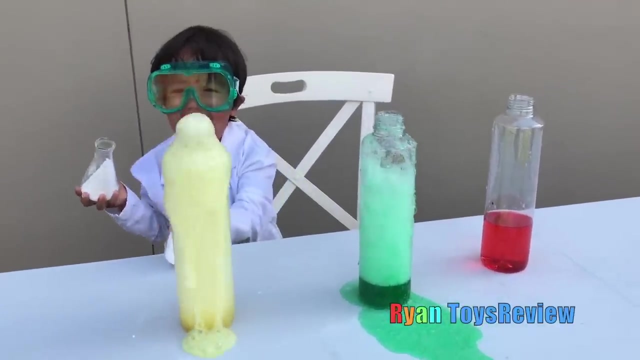 Whoa, Whoa, Whoa, Whoa, Whoa. Look, All right. Oh, that's a lot. Oh, Whoa Wait. Whoa, Whoa, Whoa. Explosion Kids. I'm gonna put quite a lot in the red one. 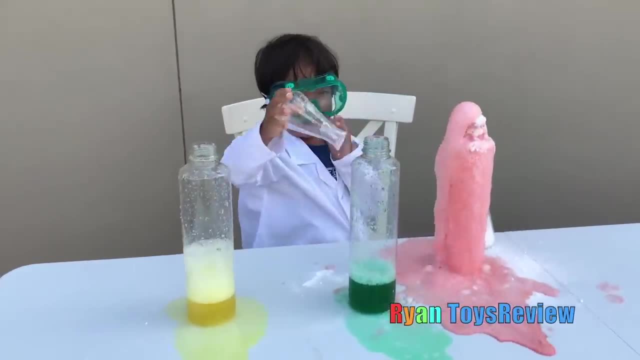 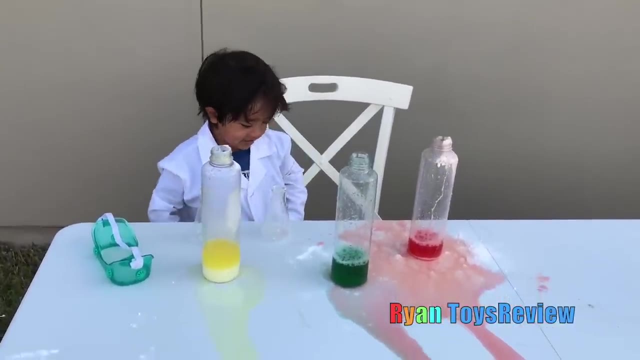 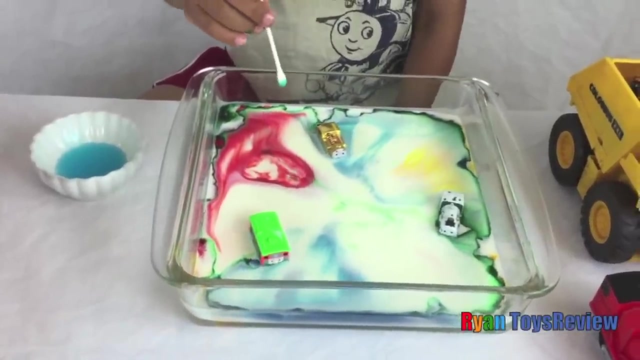 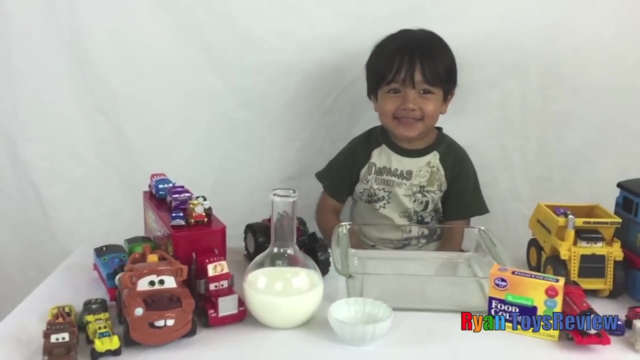 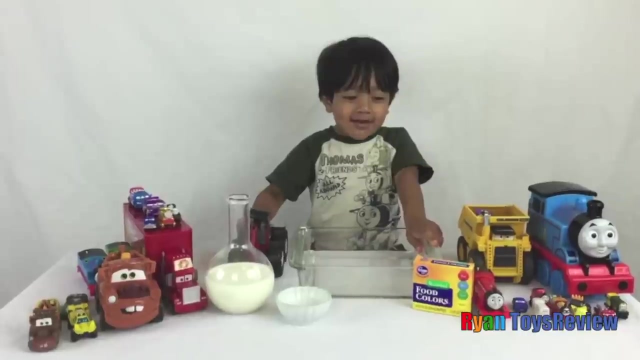 That's a bigger explosion Ready? That's a big mess. Yeah, Woo-wee, Whoa, Hi, Hi, I'm- I'm Molly. What are we gonna do today? Today, we're gonna do milk and soap experiment. 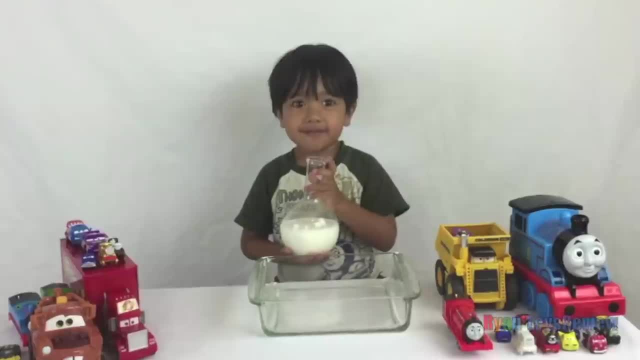 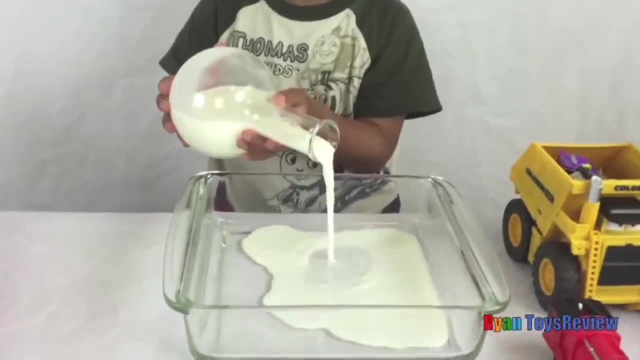 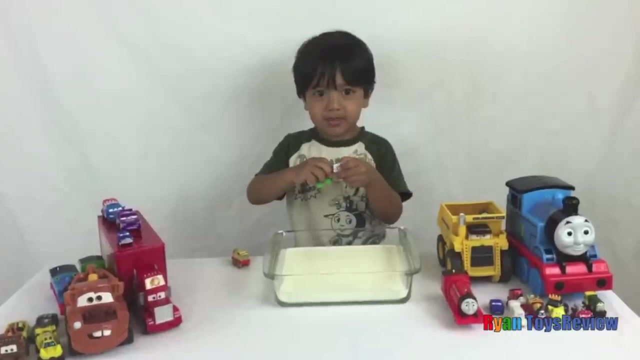 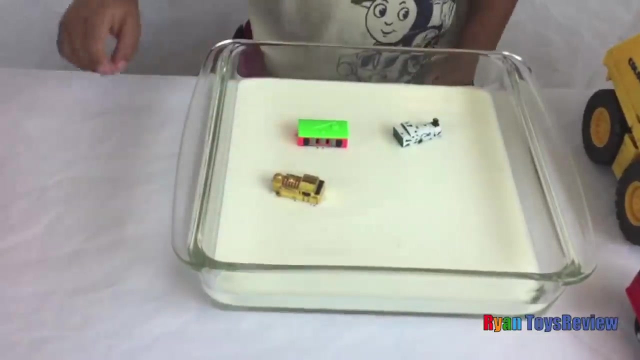 Welcome to Ryan's Toy Video. Let's fill the container of wet milk. I'm gonna put the Thomas Minis inside for fun. Chugga-chugga-chugga-chugga-choo-choo, Chugga-chugga-chugga-chugga-choo-choo. 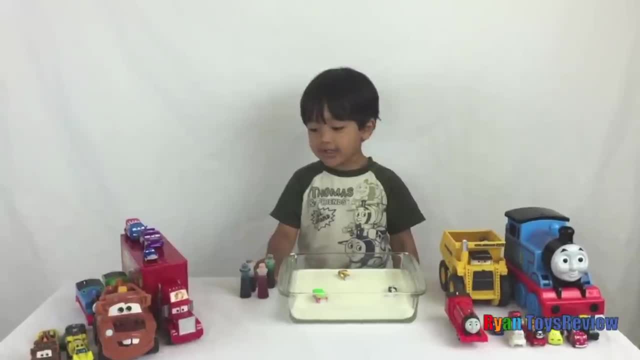 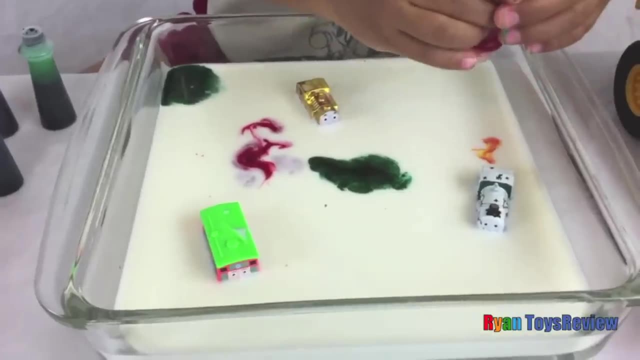 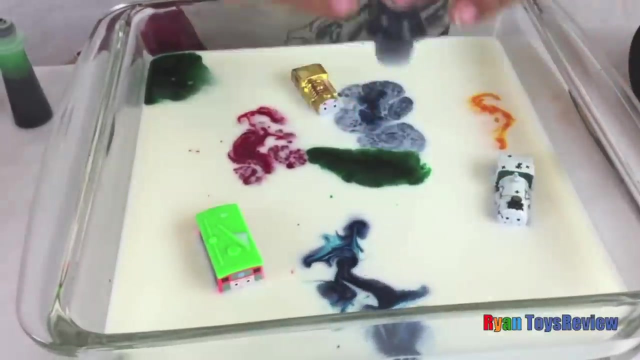 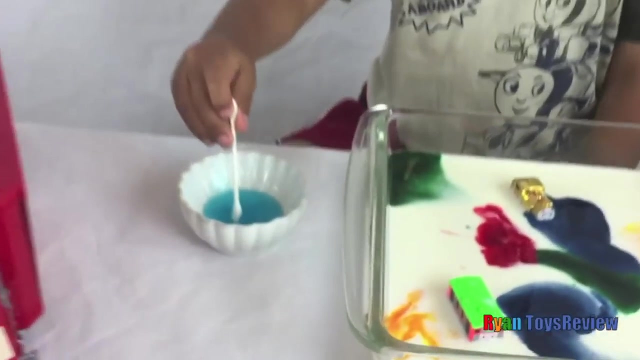 Chugga-chugga-chugga-chugga-choo-choo. Now I'm gonna add food coloring- Whoa, this is cool. Now I'm gonna dip some Yum Soap- Whoa. 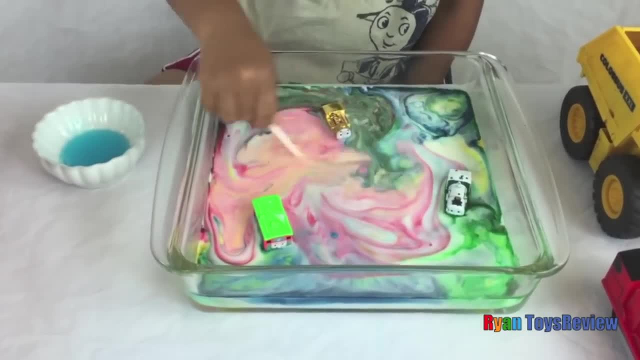 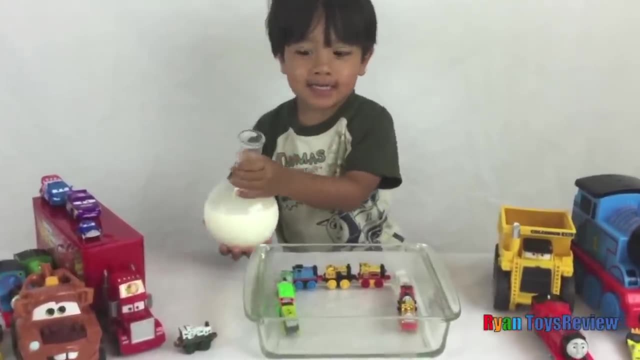 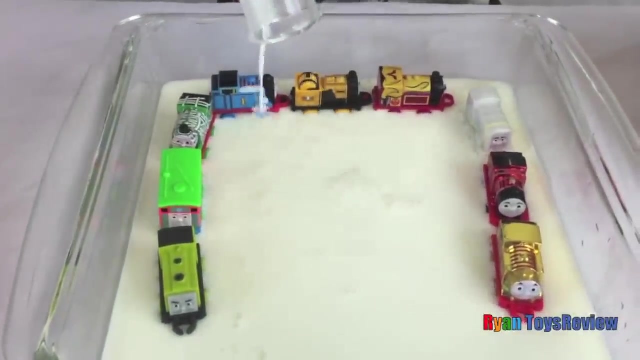 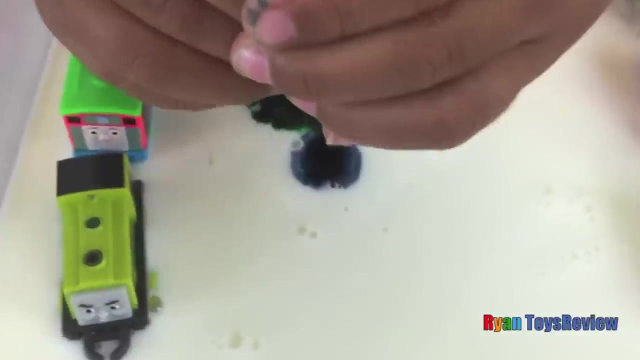 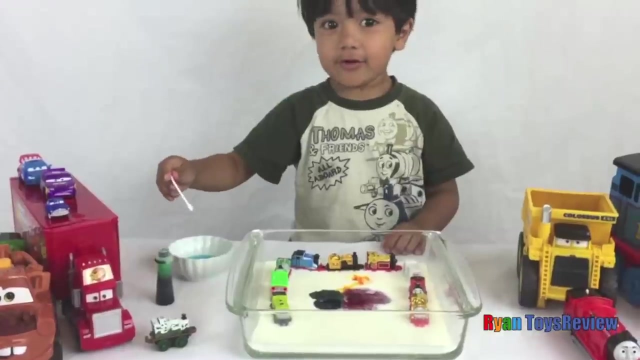 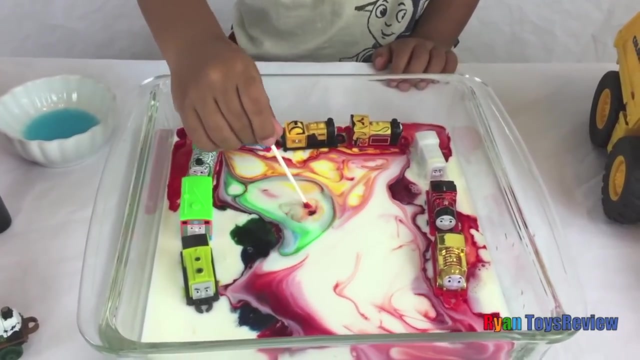 I'm gonna swirl it around. That was fun. Let's try it again. I like what happened to them. Here comes the salt. Oh, I love this. Oh, I love this, I love this. I like the taste. Oh, I like the taste. 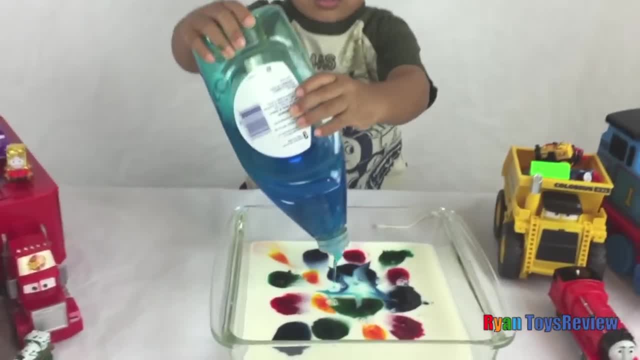 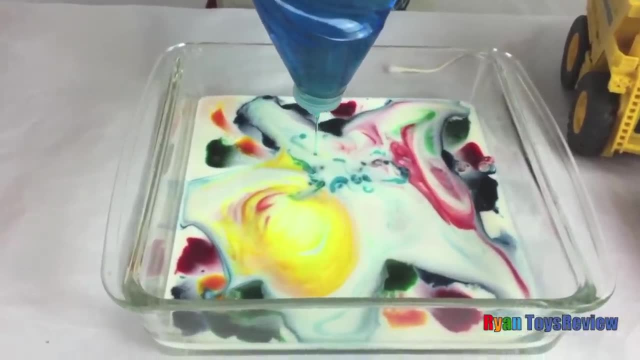 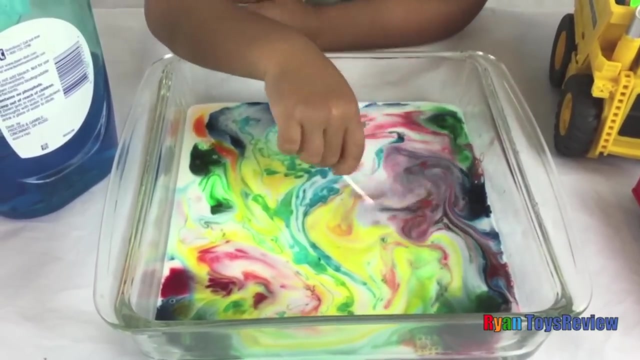 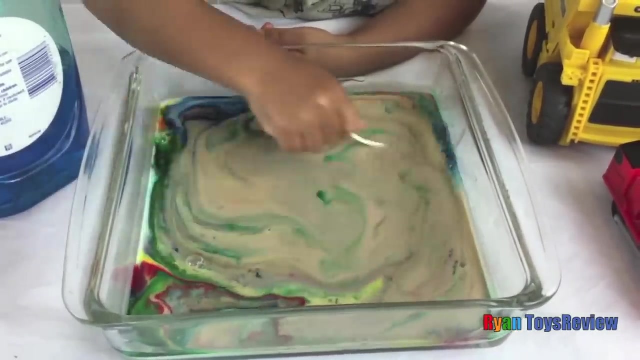 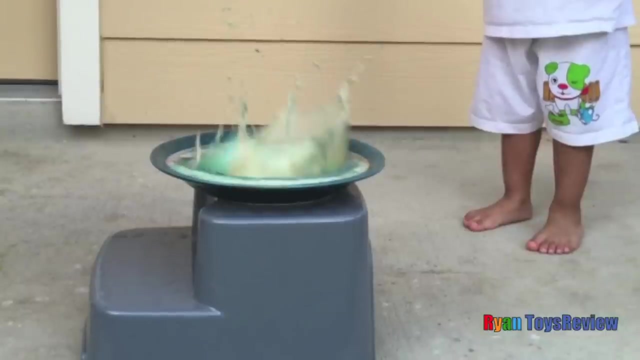 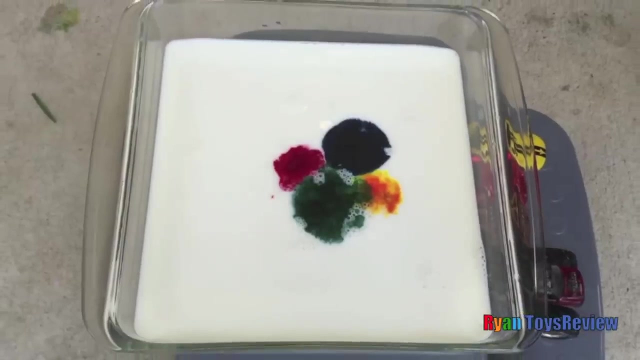 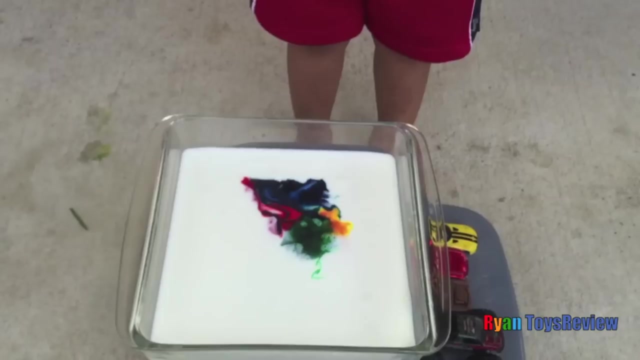 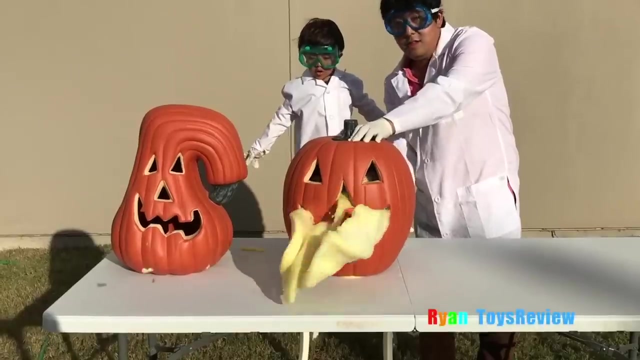 I like the taste. I like the taste. Let's stir it for fun. It's turning to brown. now I'm going to drop an egg inside. Let's drop the goat top some time. Whoa, that was so fun. you should try it out too. 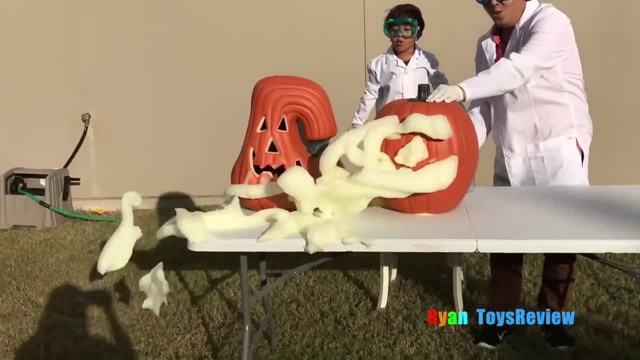 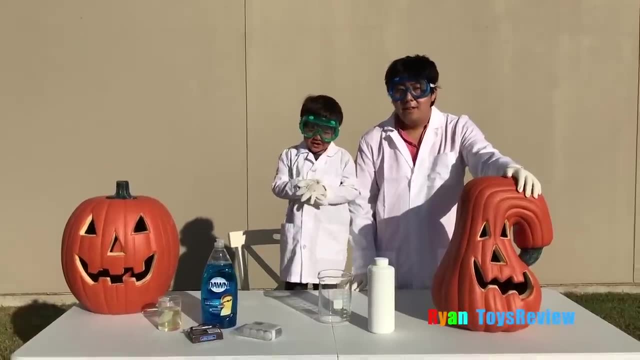 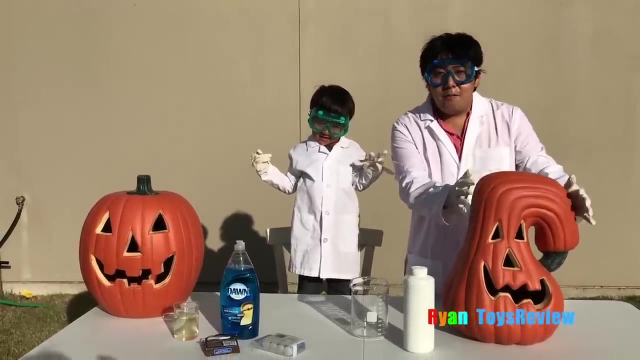 Yeah, Yeah, Welcome to our toy video. Today we're doing a grown up experiment. we're going to do the elephant with his spirit using pumpkins. That's right, we're going to do a grown up experiment first, then after that we're going. 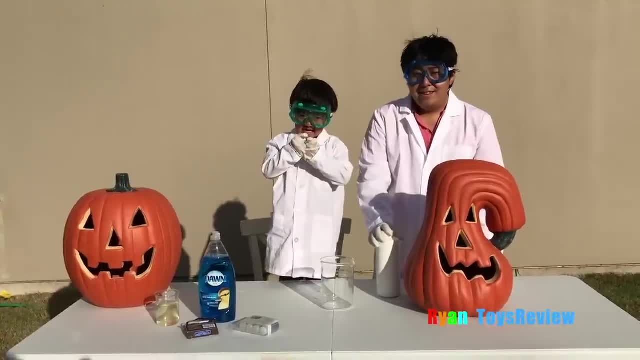 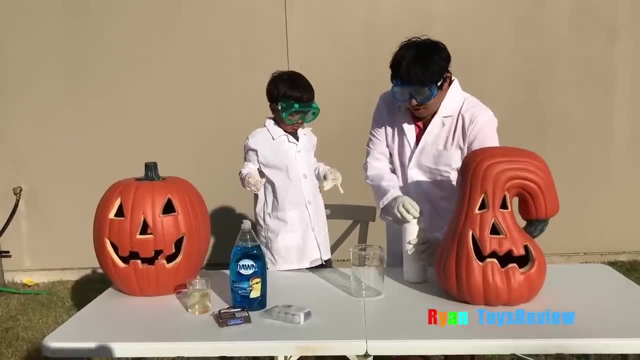 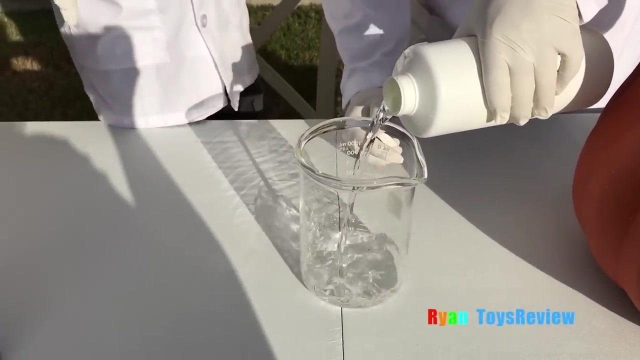 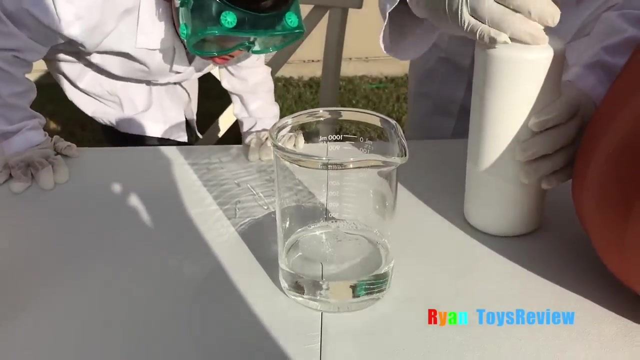 to show you a kids friendly version. So kids always ask a grown up for help and never eat any chemicals. Let's start. Alright, let's start First. we put in the hydrogen peroxide Into the beaker. Okay, that's enough. Next add food coloring. I'm going to use yellow. 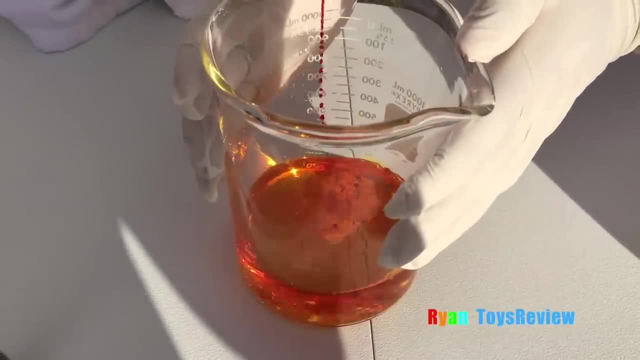 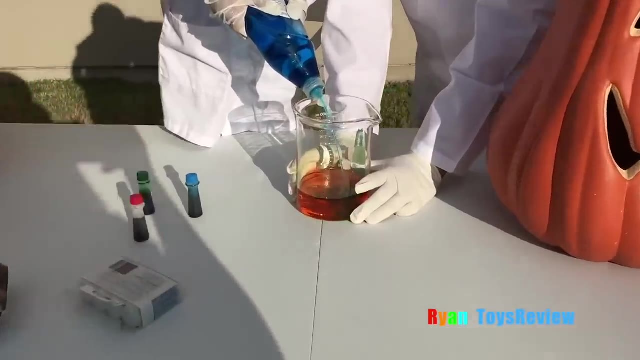 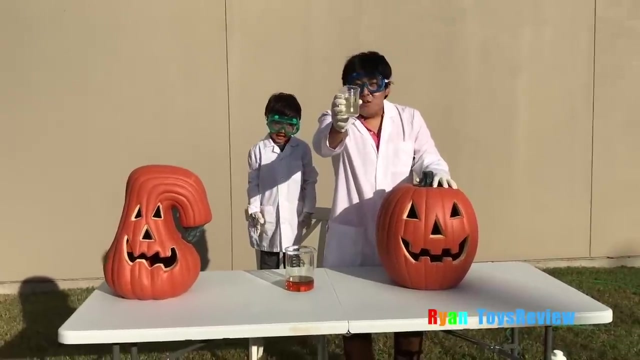 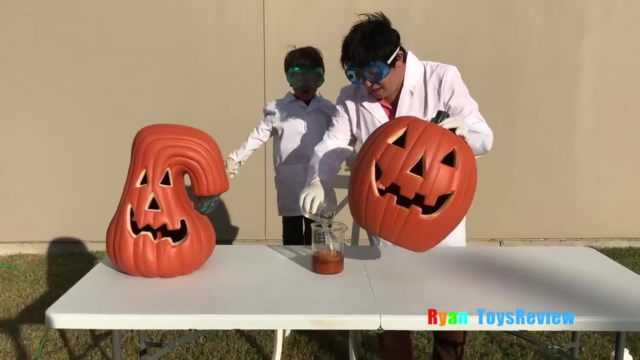 Oh yeah, it looks yellow Good. Next let's add some strong soap. All right, all right, that's good. Thank you, Looks cool. Okay, this is a catalyst. It will speed up the chemical reaction. All right, you guys ready. There's so much. 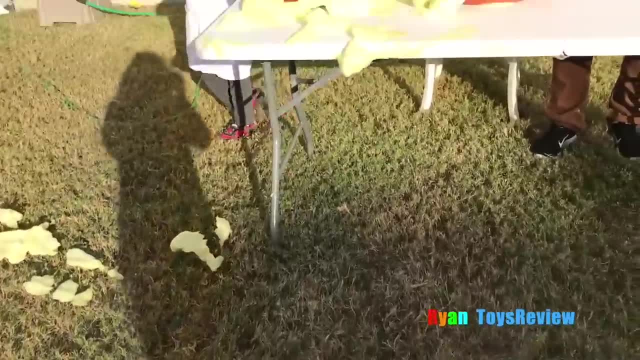 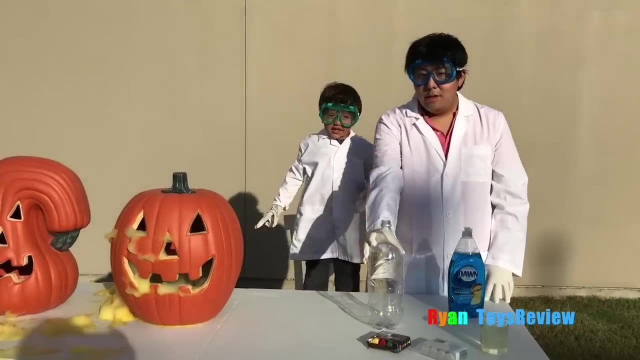 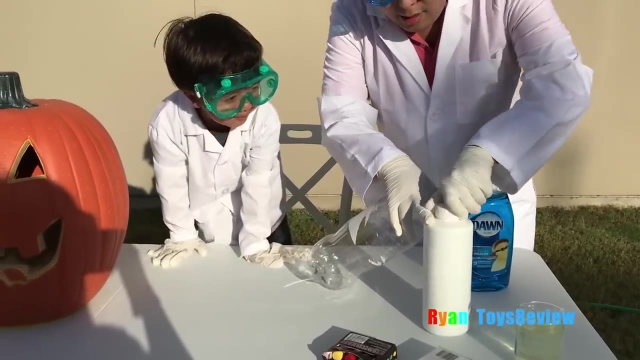 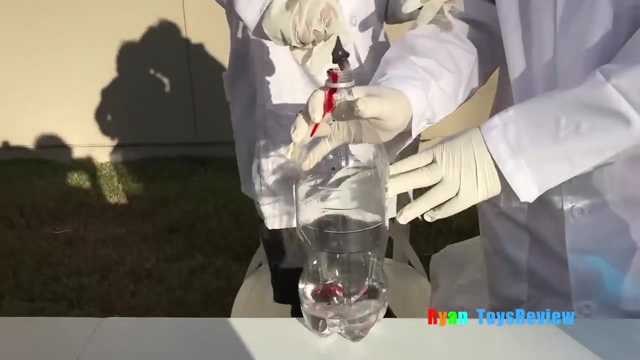 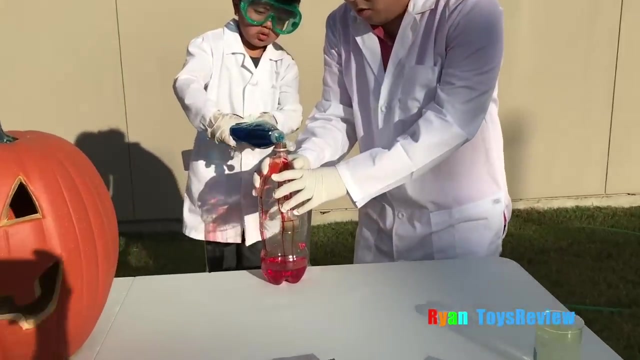 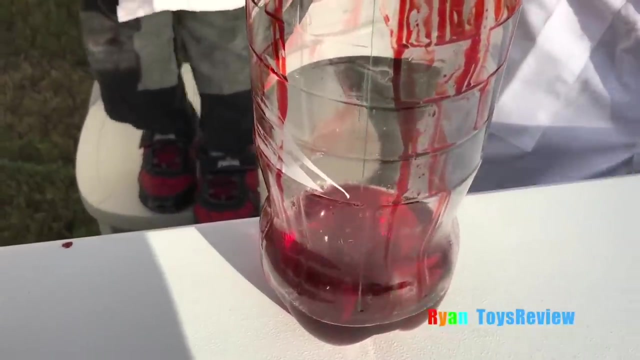 Everywhere, Did you see? Now try again without the pumpkin. All right, again we're gonna put hydrogen peroxide Soap. Yeah, we use soap to trap the gas. All right, now let's add the catalyst. You guys ready? Yes, Let's see in action. 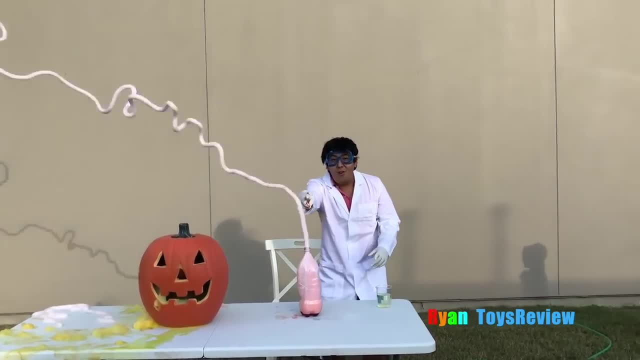 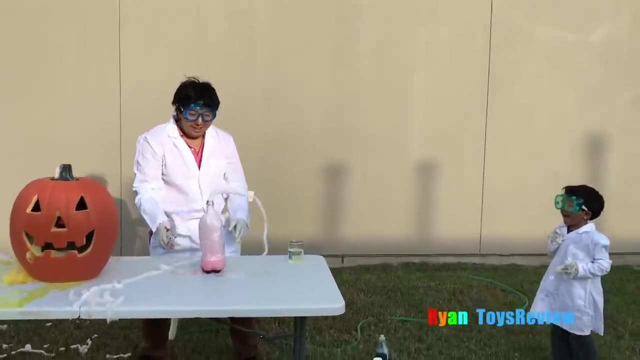 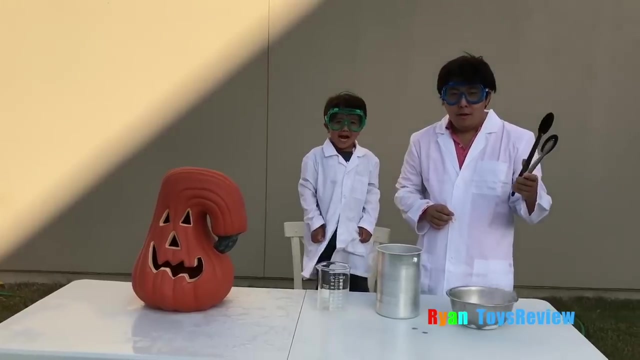 Whoa, look at the hens, keep going. They're going. Whoa, Whoa, Let's keep going. Look at our yard, Ryan. Look at this. Oh my god, Now we're gonna have fun with our hens. We're gonna have fun with dry ice. 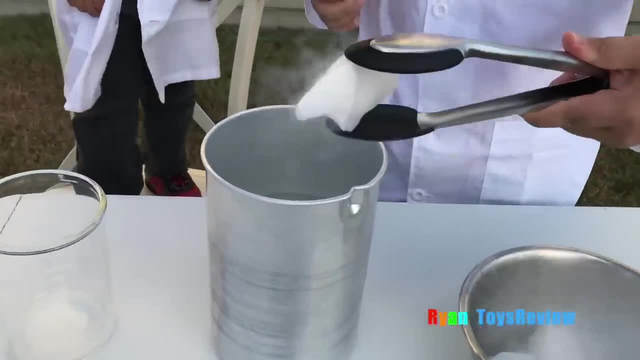 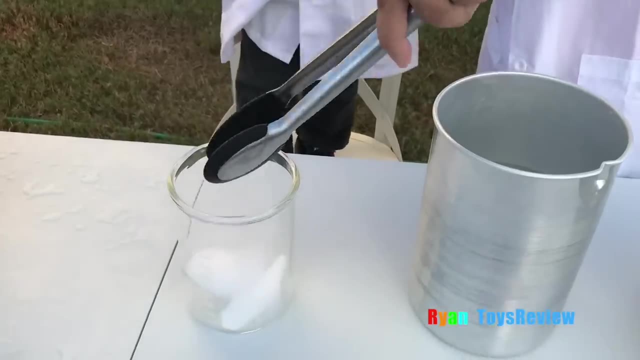 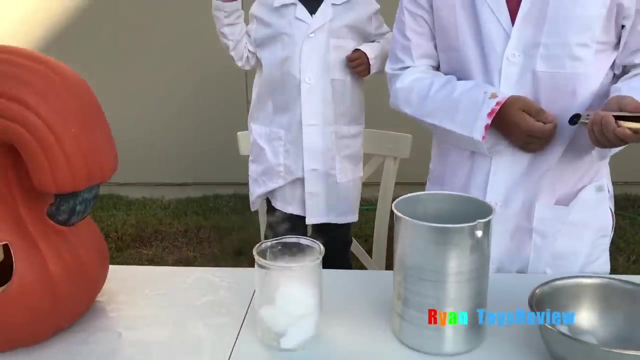 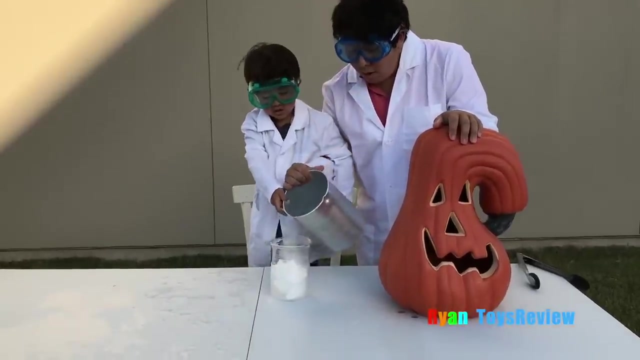 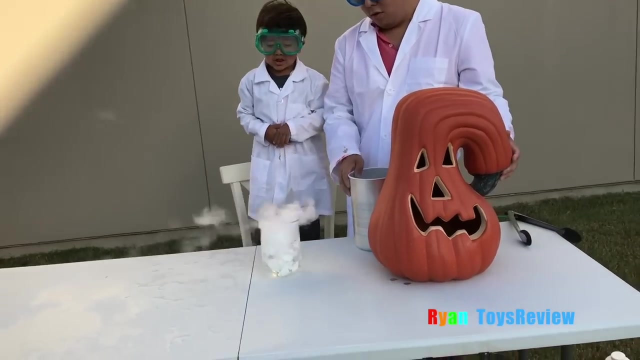 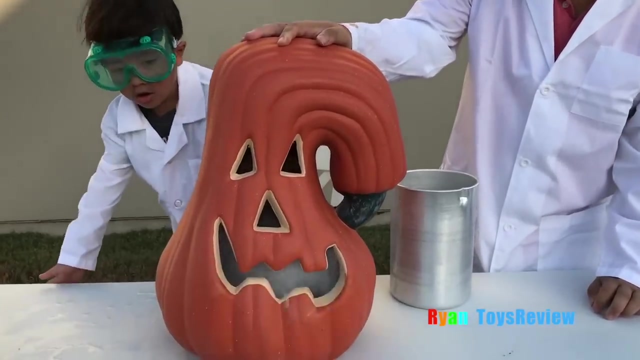 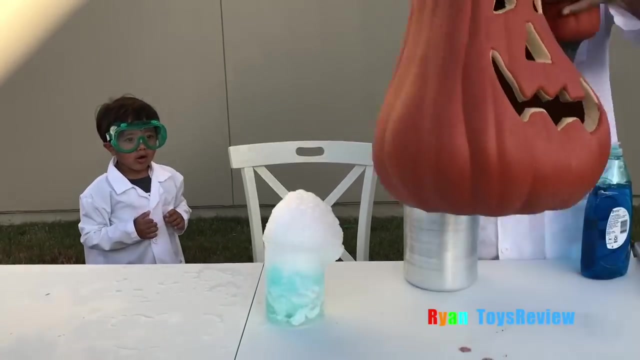 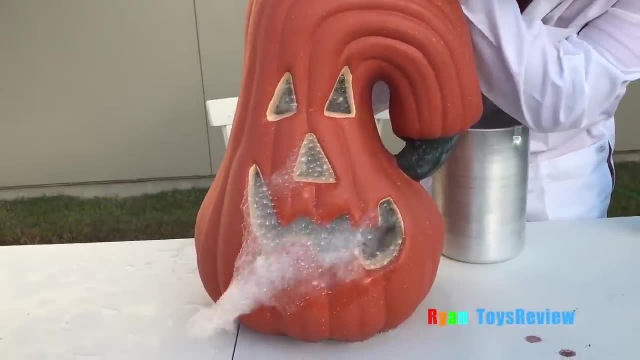 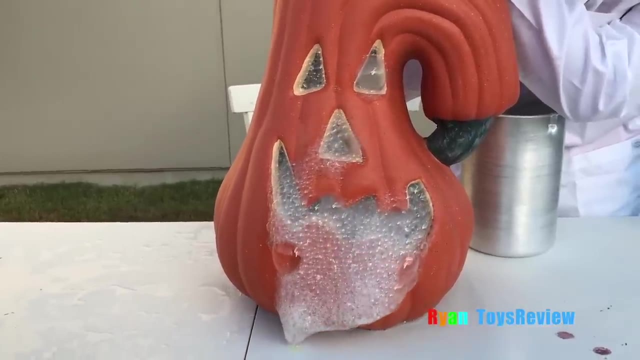 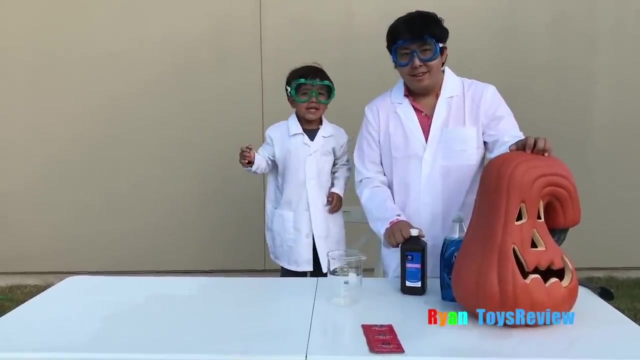 Whoa, Woah, It's so cold coming out from his mouth and nose and eyes. whoa, now we're gonna do the elephant toothpaste kid friendly version. that's right. for this version, we're gonna use a hydrogen dioxide. that's only three.